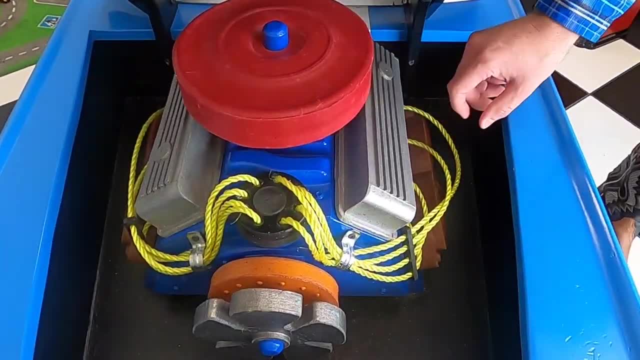 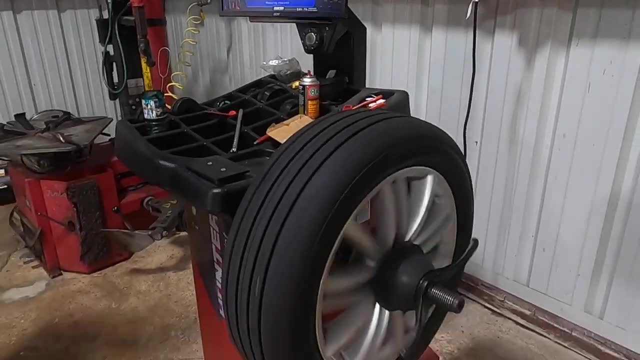 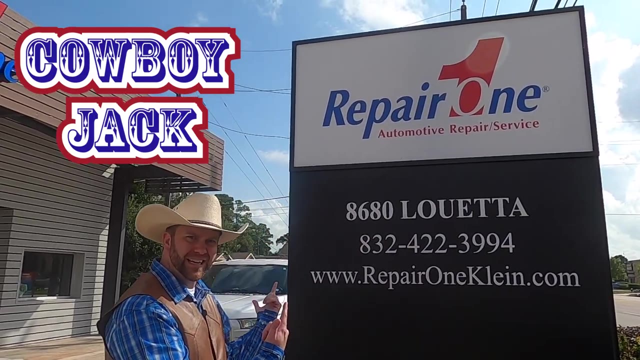 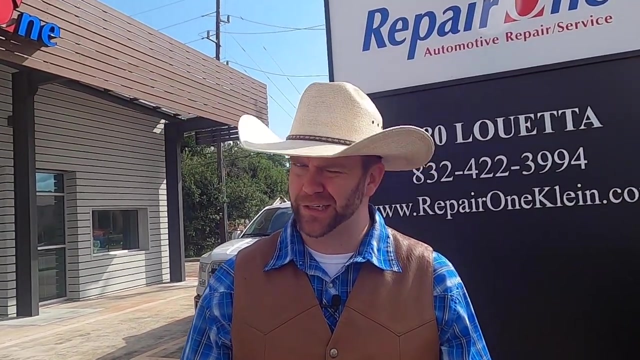 Howdy, cowboys and cowgirls. I'm Cowboy Jack and I'm real excited. Do you see where we are today? Take a look at that. We're at Repair One in Spring, Texas. You know, sometimes when you're driving around in your car, well, you guys shouldn't be driving yet. that's silly. 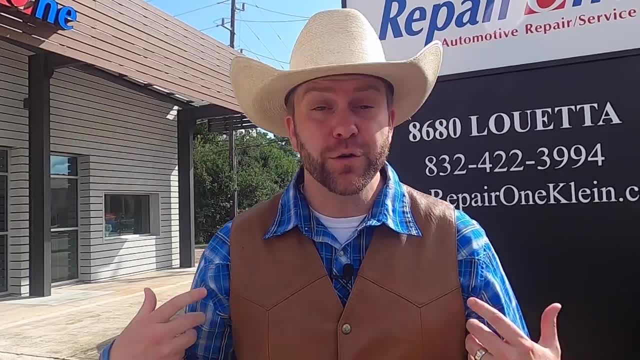 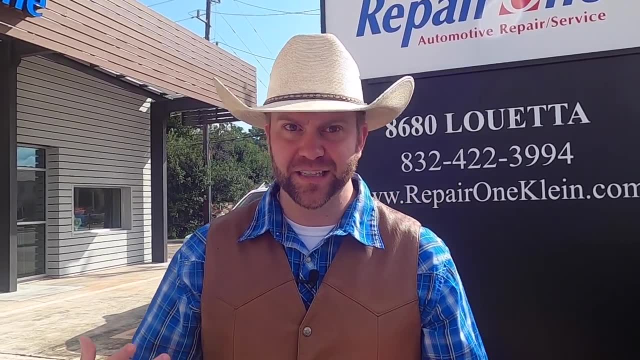 When your parents are driving around, you might need a repair on your vehicle and bring it to an auto shop. That's where we are today. Have you guys ever been in an auto shop before They're going to? let us look all around and see what it is they do all day It's going. 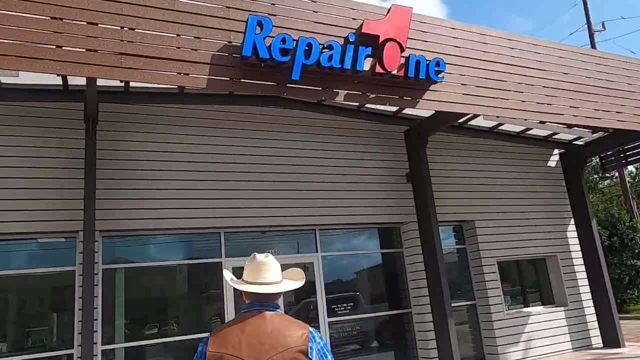 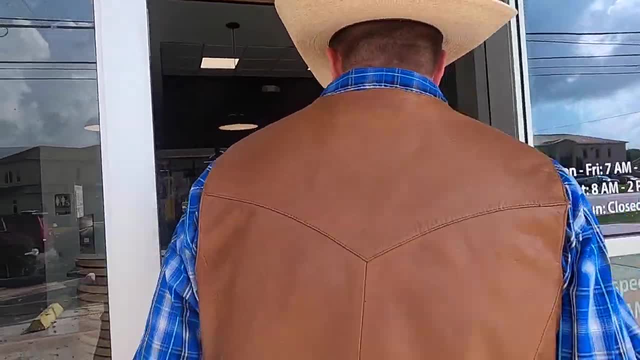 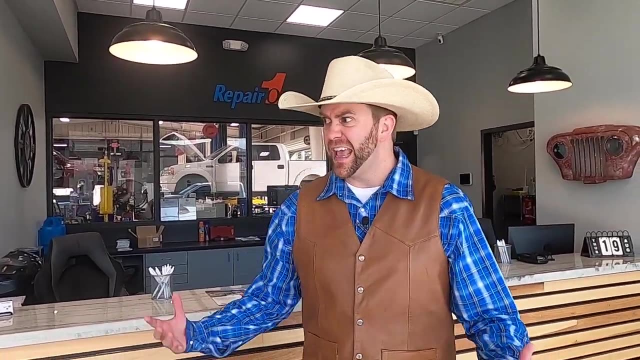 to be really cool. Alright, come on, let's go. Wow, this looks like a brand new building. This facility was just recently done. Really cool. Wow, it's so clean and nice in here. Everything looks great. They have a really fun waiting area. Come on, let's go check. 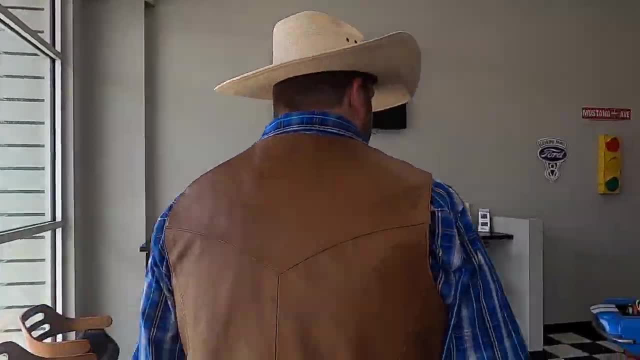 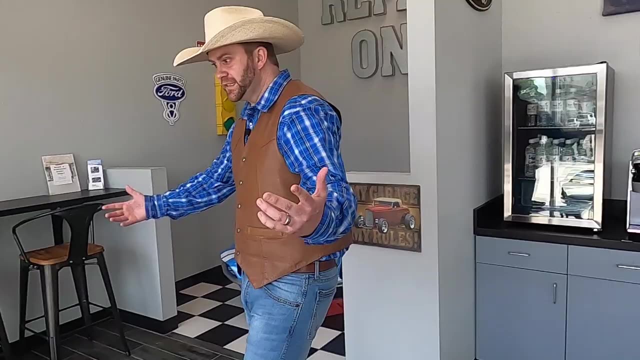 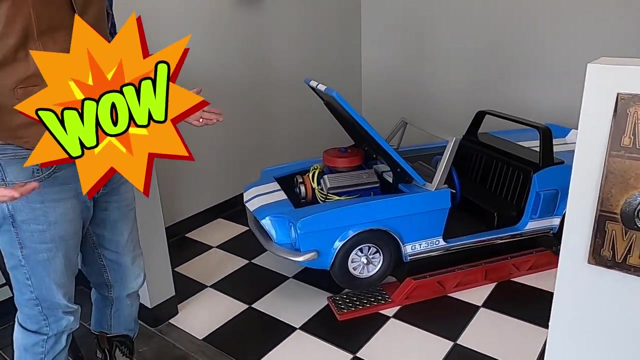 it out. Wow, this is cool. It looks like they've got some coffee for adults, some water for us and they've got magazines and all kinds of things. Whoa, guys, come here and look at this. They have an actual play area in here. That's really cool. So when you come, 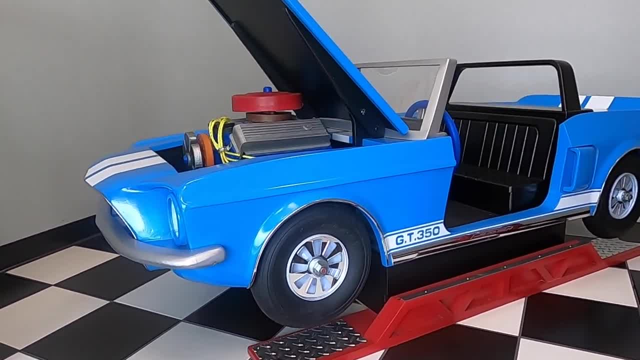 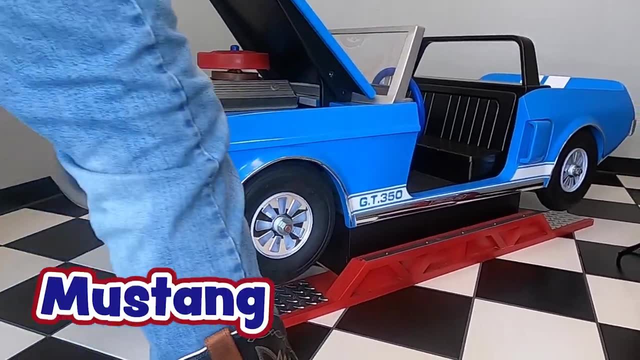 here with your parents and you're waiting on your repair. you can actually come in here and play with these things. This is a Shelby GT350.. That's a cool, cool Mustang. They actually have a little miniature one in here and it's got all these engine parts and everything. This would be like the. 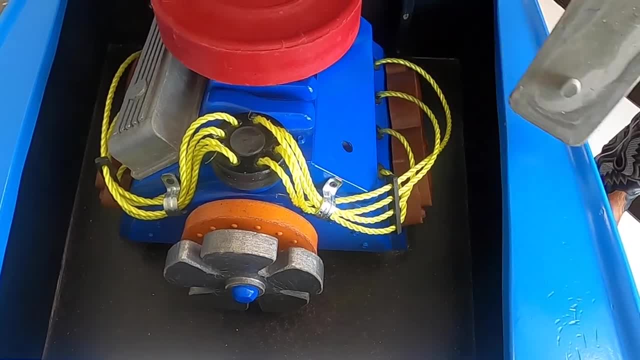 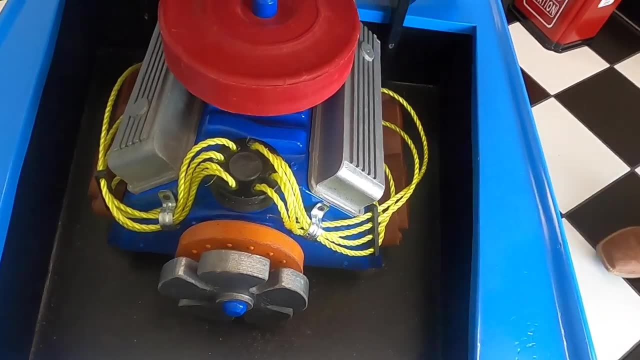 air filter right here. This would be your Whoa- they even come off. That would be your valve covers. Let me get it back on there. That is so cool. You can play with that whole engine and there's even some little cars and trains over there to play with- and a real 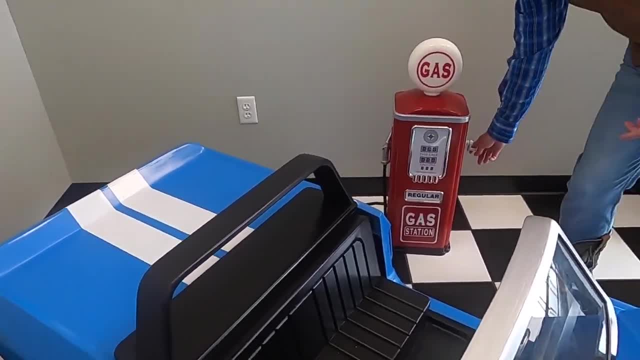 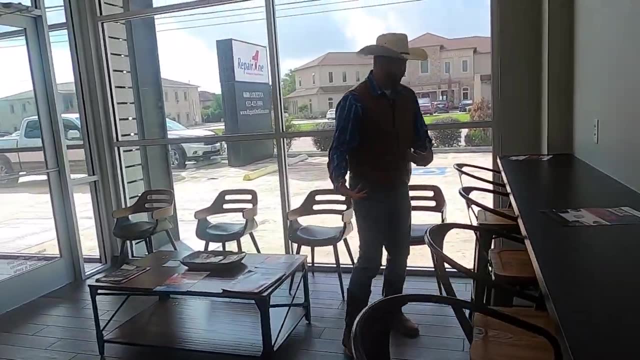 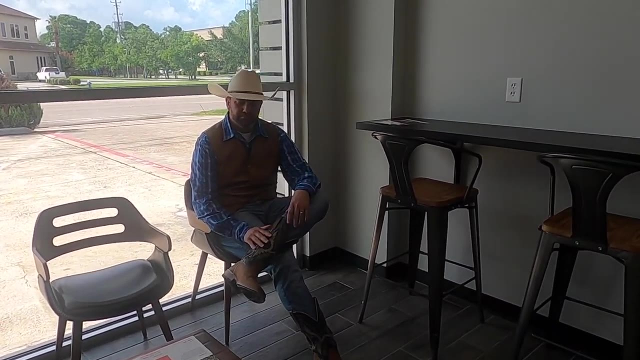 old-fashioned gas pump. Wow, That is so cool. Well, so when you're waiting on your parents' car to get fixed, you can either be in there playing, or you could sit down right here in a chair and wait for the car, All right, Well, you guys know what it looks like to wait, right, If you're? 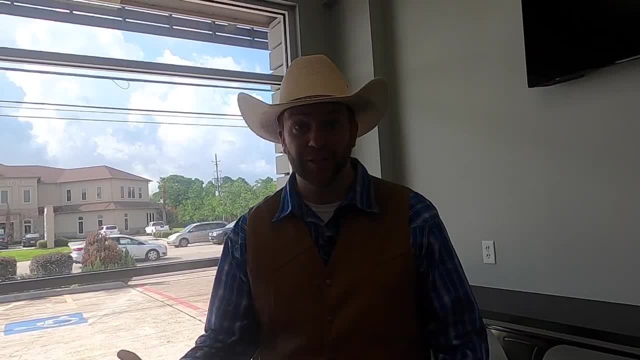 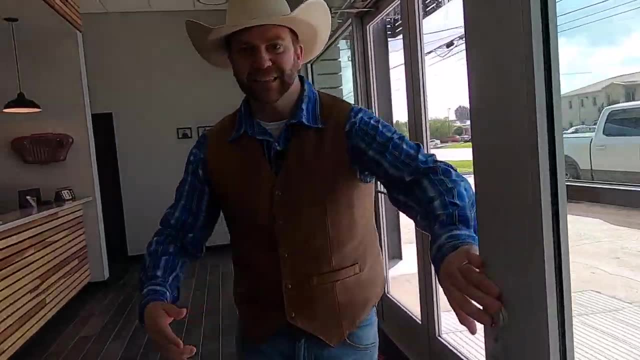 waiting. you've got to act real good and be patient because they're working hard out there. But anyways, let's go take a look inside the shop. Come on guys. Oh wait a second. Look who it is. This is my buddy, Brian. Hey, Brian. 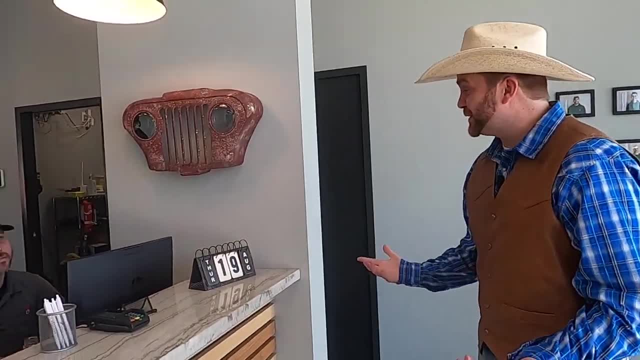 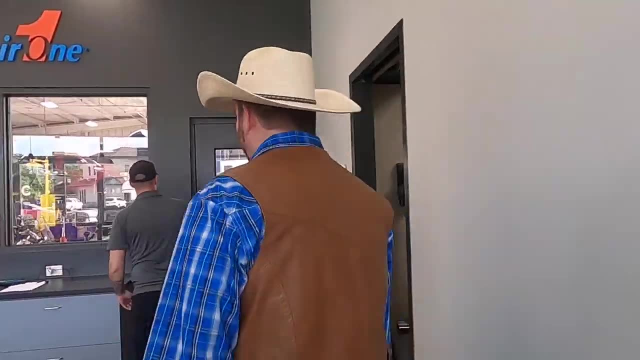 how's it going? How you doing today? Good, good, Hey, would it be okay if we took a look outside in the shop? Absolutely, Let's go this way. All right, Come on guys. He said: yes, we can actually look in the shop. Whoa, This. 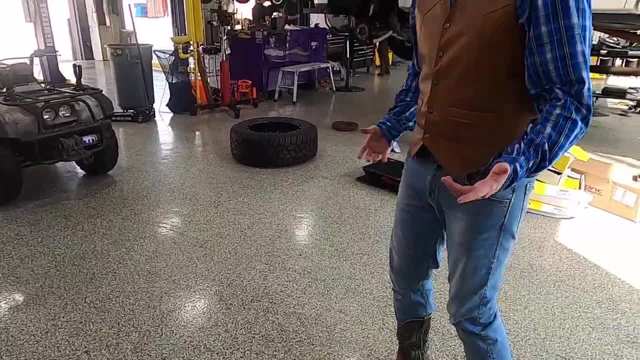 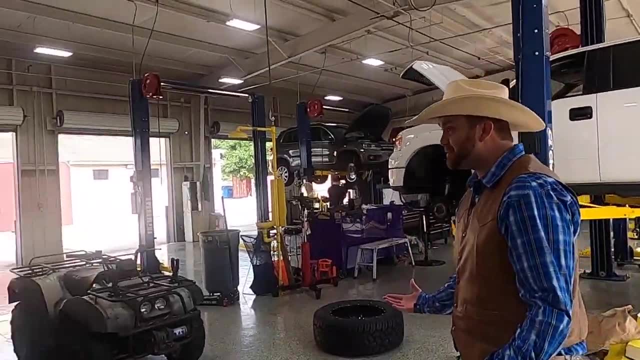 is a really awesome shop. I mean, guys, this is where they work on cars. Take a look at the floor. It is spotlessly clean. You guys must work really hard to keep it clean in here Every day. Wow, that's great. You could even eat off of this floor. I'm not going to, but I'm saying 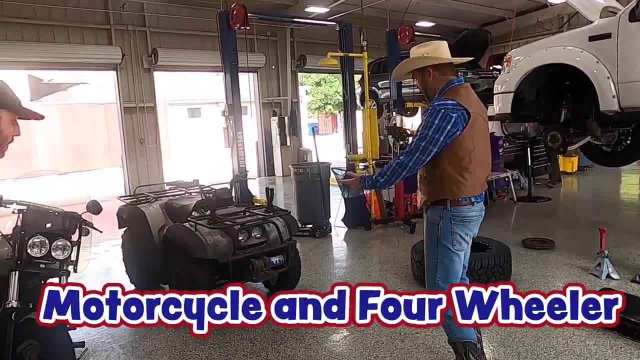 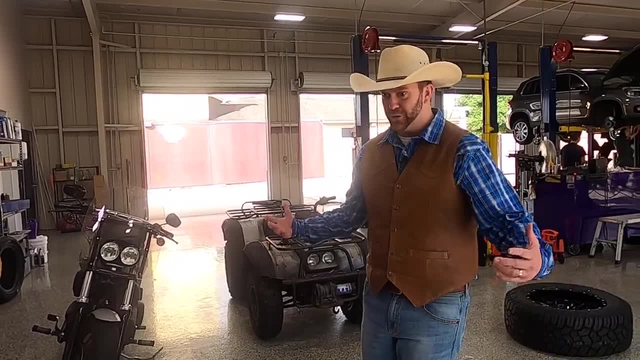 you could if you wanted to. Wow, here's a motorcycle and a four-wheeler. You guys work on those too. Everything that's got tires, Everything that's got tires, That's so cool. So anything that's got tires that's got a. 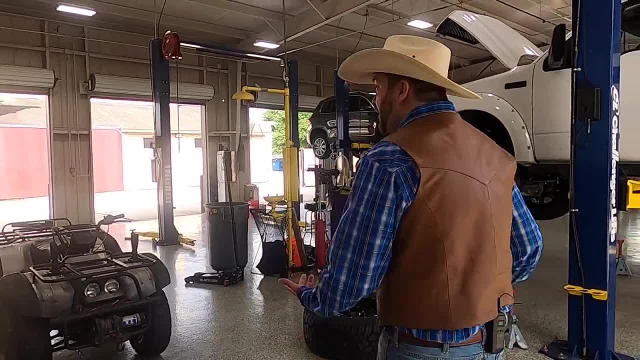 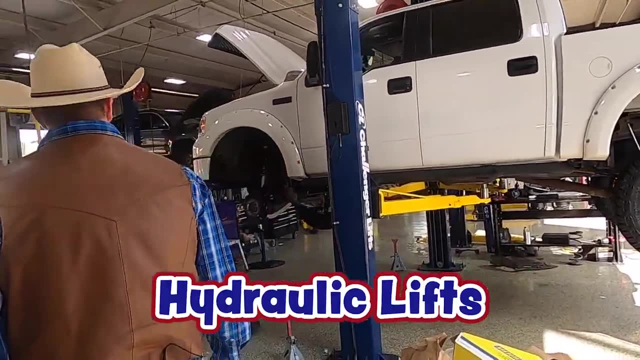 problem. you could bring it right here. Wow, I've always wanted to know what are these big things that lift up the cars? Those are our hydrogels, Hydraulic lifts. That way we can get underneath them and do any work underneath we need to. 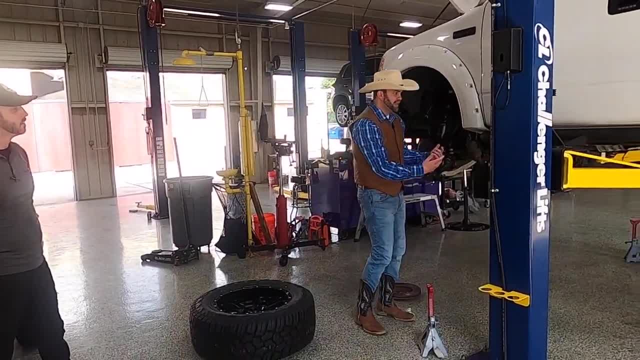 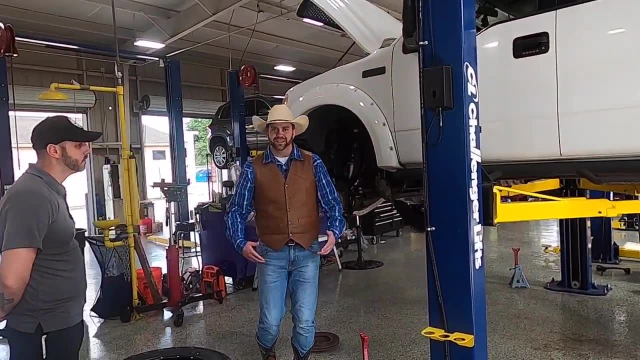 Wow. So I guess you would pull up a truck in here and move these different arms underneath there and it just lifts it right up, Absolutely. And they work with hydraulics. Yes, they do. It seems like a lot of things that we talk about work on hydraulics. You guys remember. 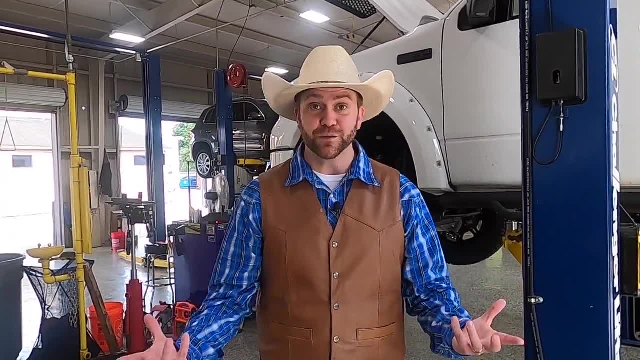 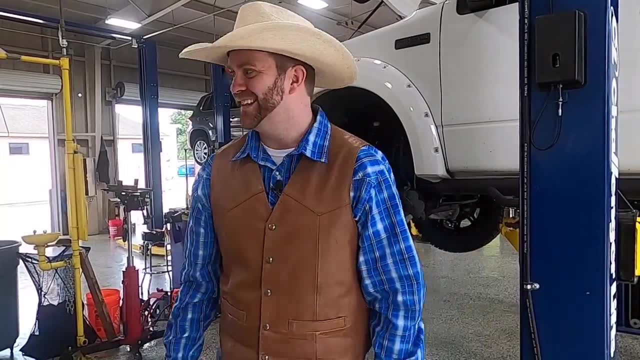 about hydraulics. Hydraulics is something that uses hydraulic fluid and a series of compressions and release valves to make things move. It's really cool and really strong. Hey, Brian's actually going to operate the lift for us so we can see what it looks like. 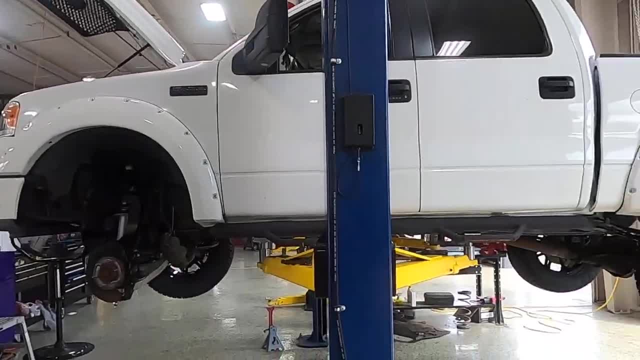 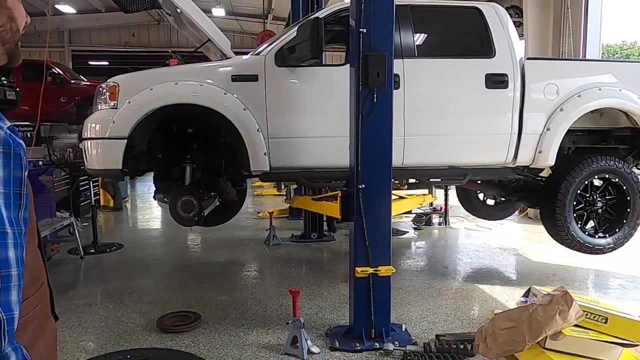 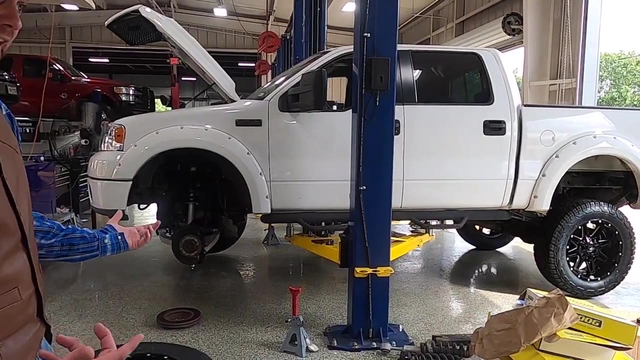 when a vehicle goes up or down. Guys, take a look. Wow, he's bringing it down, Seeing right now that hydraulic system is open, so it's releasing the fluid and it's letting it come out. Now he's going to close that valve and it'll lift it right back up. 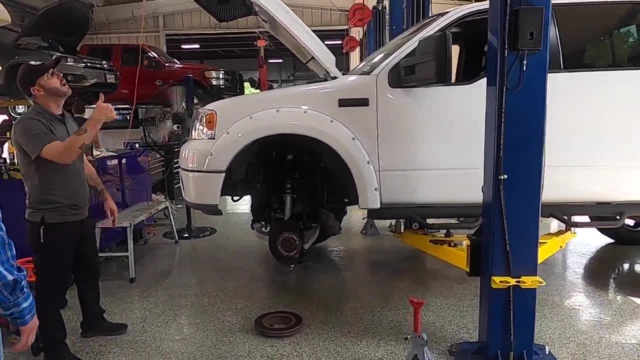 Okay, so it'll start like this and then I'll show you how high it'll go. It'll go all the way to the top. Oh wow, It's going to lift the lift up. I like that. I like that It's going to lift. 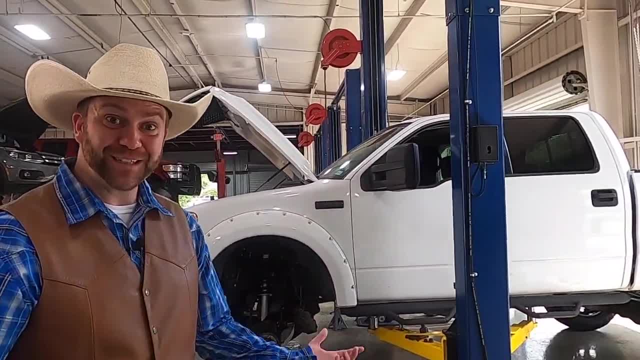 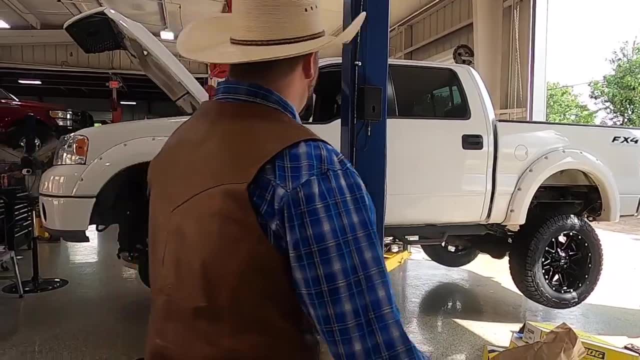 Oh wow, He's going to lift it all the way up to the top. That's going to be so fun to see. I mean, how much do you think a truck weighs? It's not light. This machine works really hard. 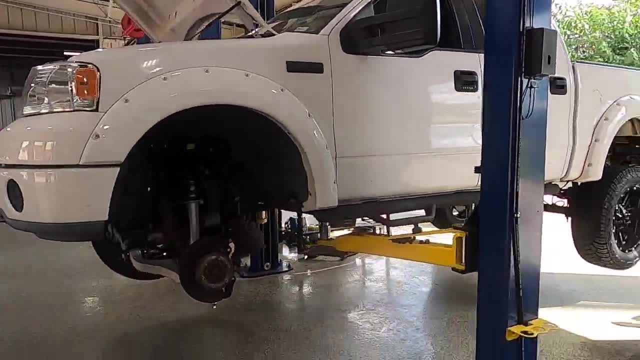 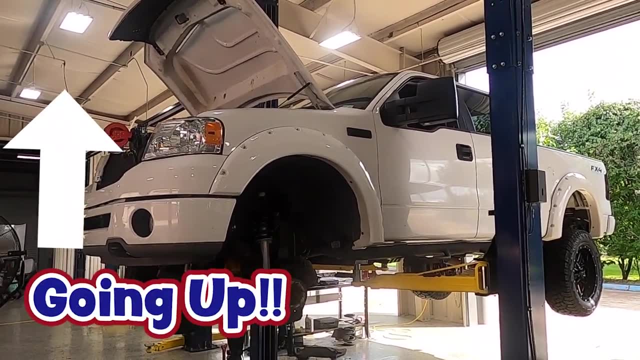 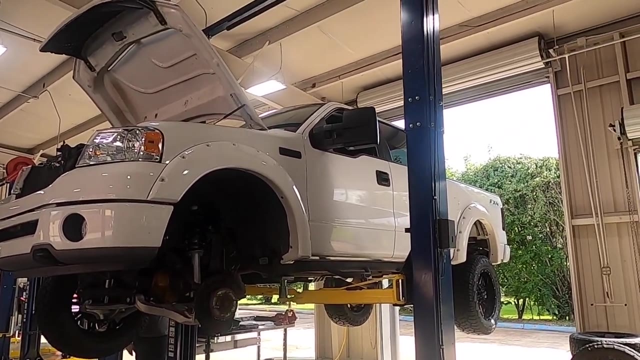 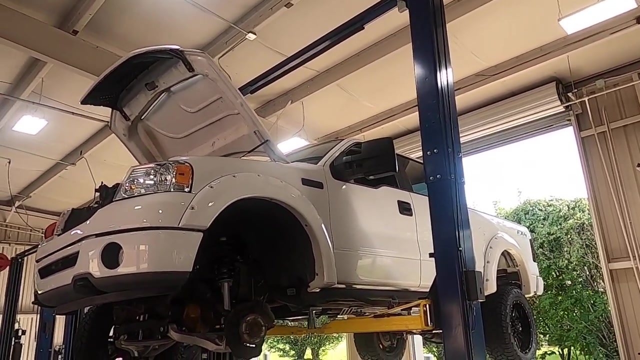 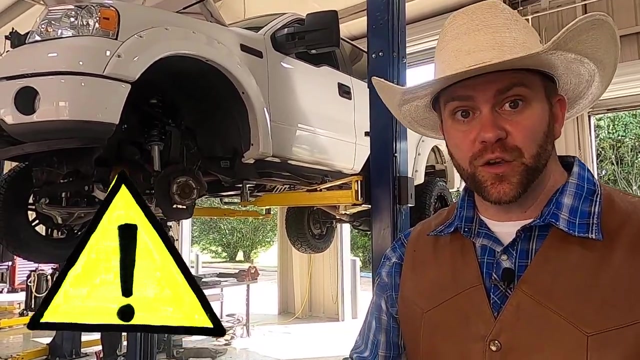 Wow, That is going really, really tall. That's crazy. You guys hear that loud clicking noise as it's going up. What that is is a system. It's a safety release. So whenever it goes up past a certain point, a little lever falls down. 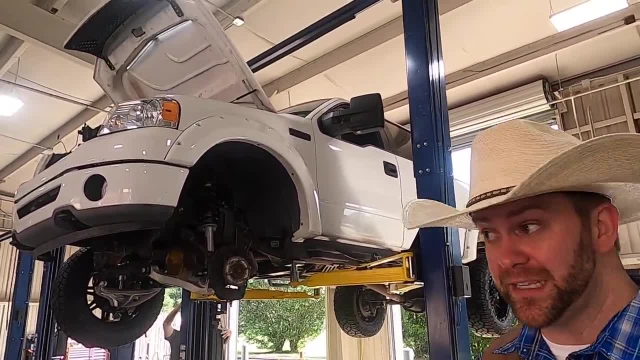 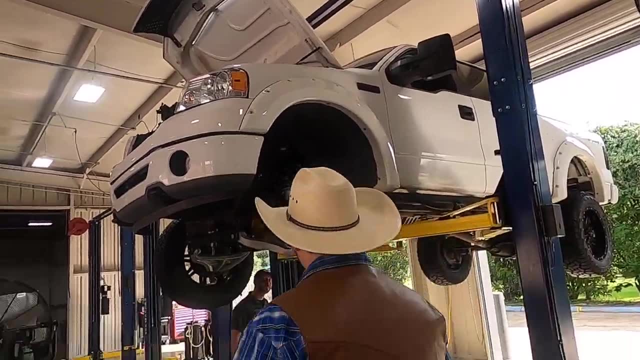 so that if the hydraulics failed, the car wouldn't come down. It's locked safely in place. Wow, That's up really high, That's super high. Wow, You could even come in here. So this is what mechanics do. Come on, guys, Come here. 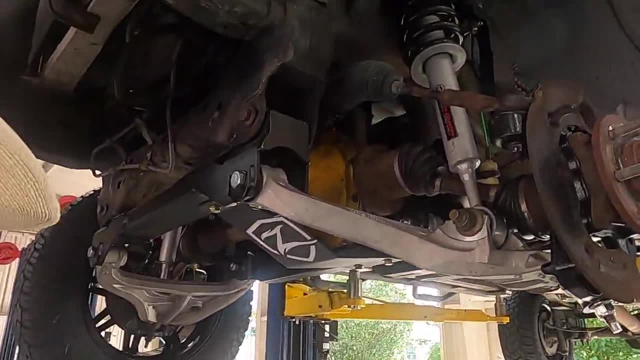 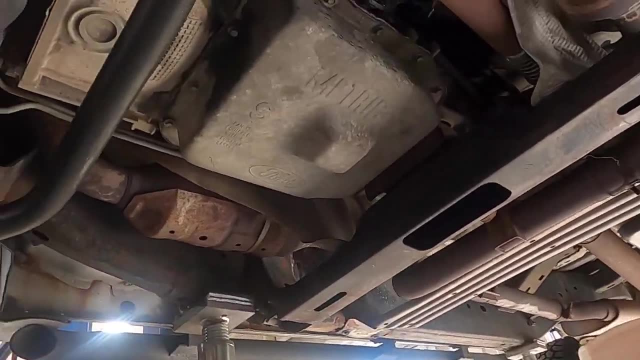 So once it's lifted up, you can go underneath there and work on all kinds of things. huh, Absolutely. So wow, Have you guys ever seen underneath? I mean, I don't know all the parts, Brian could probably tell me, but I know the engine is right here. 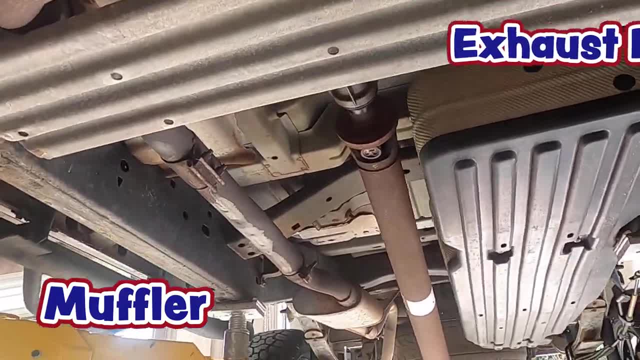 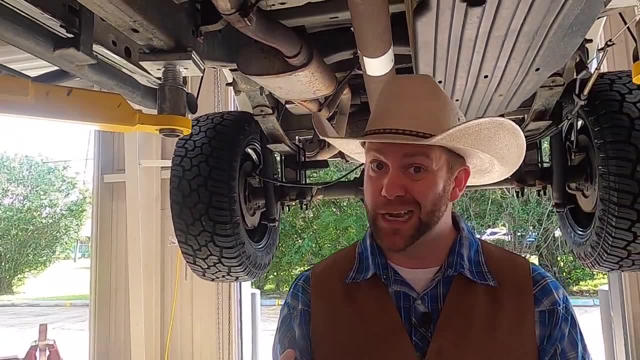 And then look, it's got the exhaust pipes and the muffler. There's probably a catalytic converter around here. There's a whole bunch of parts, but we didn't come to learn all the parts of an engine. Cowboy Jack doesn't even know that. I just wanted to show you guys that lift. 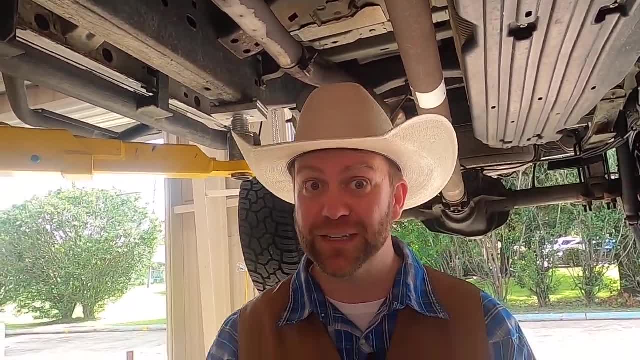 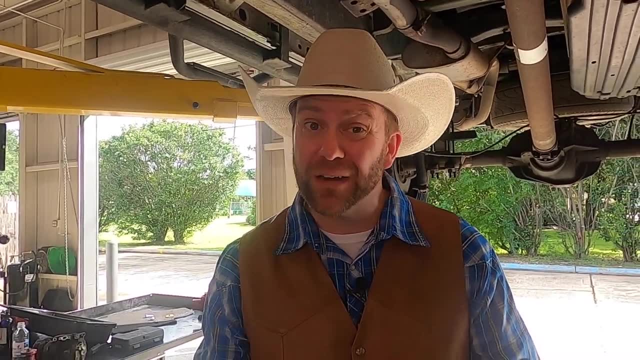 That's really really cool. Wow, All right. Well, for safety reasons, let's get out from underneath the vehicle. Whenever you're here, you wouldn't come out into this part. It's going to be really dangerous. It's not made for kids. 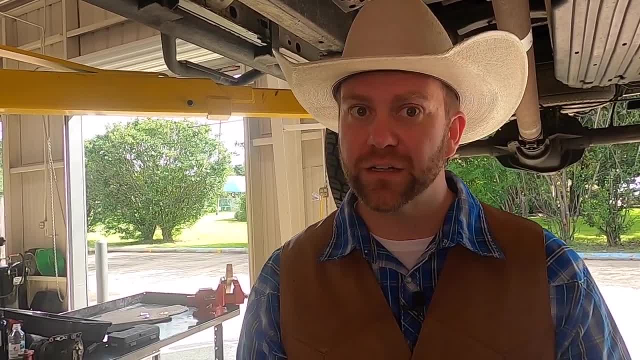 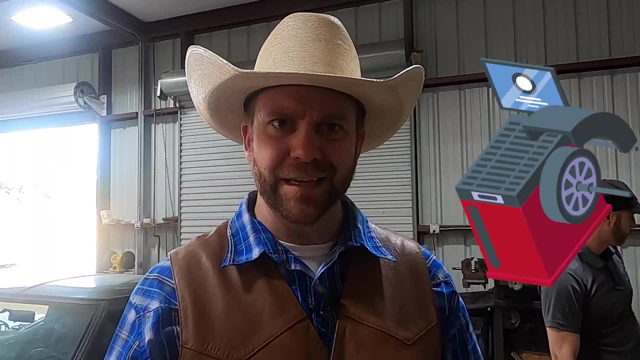 We're just taking a behind the scenes look and you would never want to walk underneath the vehicle, So let's get out of here. Did you guys know that every once in a while you have to balance your tires? That seems silly, but a tire is round and it spins around really fast. 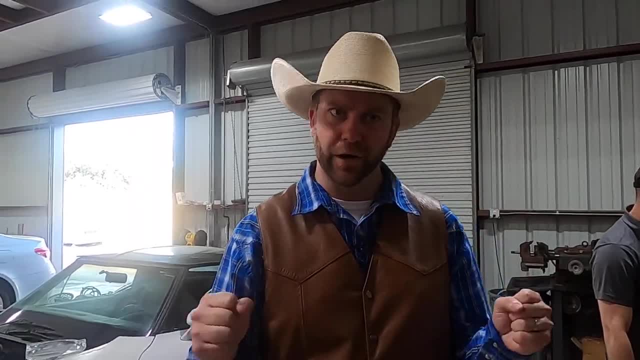 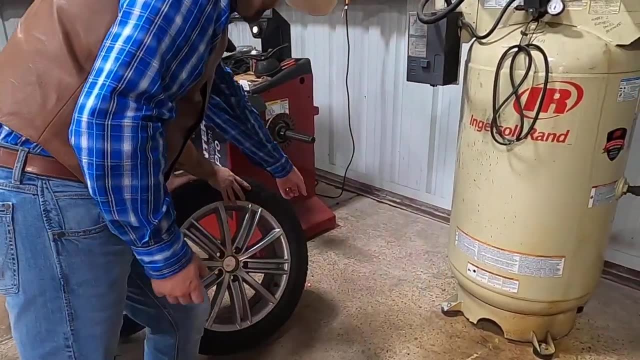 So you want it to be nice and straight and balanced so that it doesn't wobble, and give your car a little shake. Brian here is going to show us the tire balancing machine. This is really cool. Wait, wait, wait. What do I see right there on the ground? 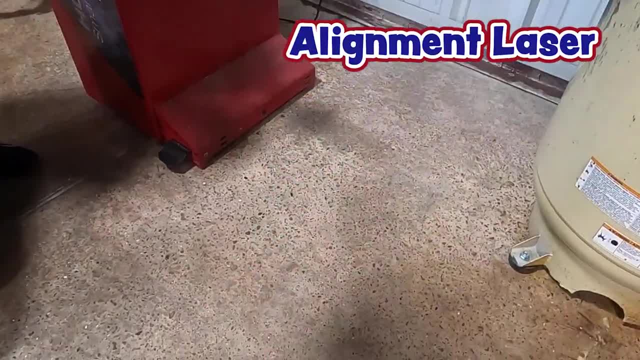 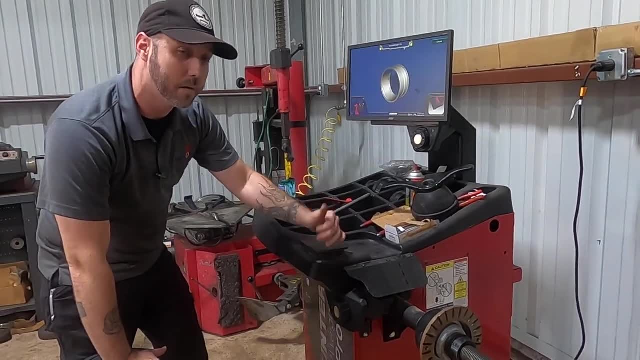 This is going to be the alignment laser. So once we get the tire on, you'll see right here this controls the laser. We'll have to put in the specific measurements of this rim in order to get the right measurement for the tire balance. 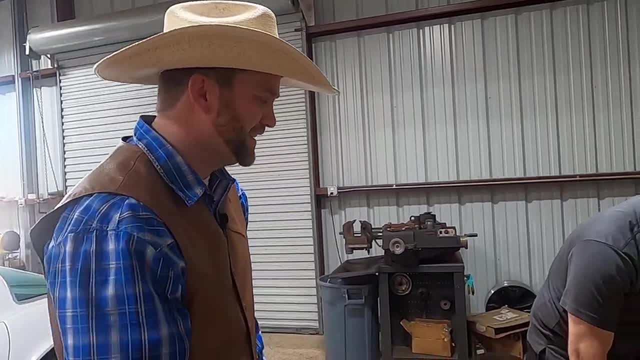 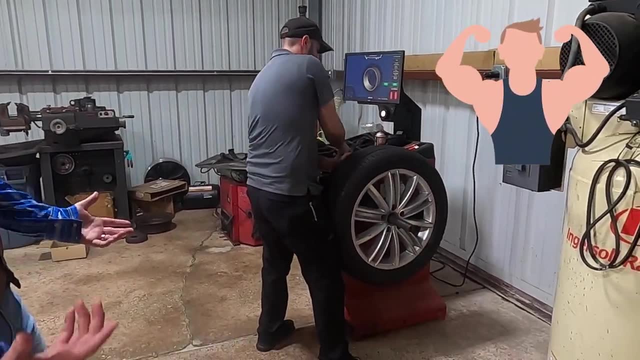 Wow, that's really cool. You even use lasers to balance tires. Absolutely All right. Brian's putting that tire on the tire balancing machine, like we talked about, And we're going to see it spin and he's going to show us what they use to balance it. 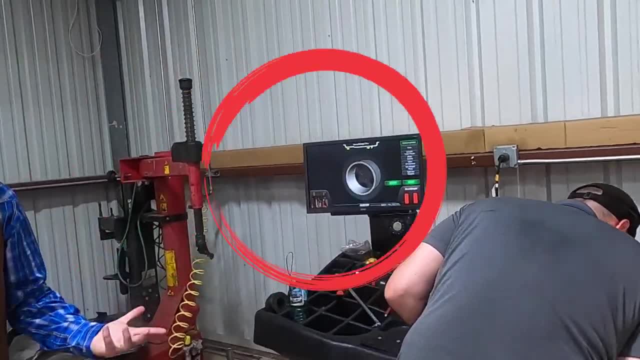 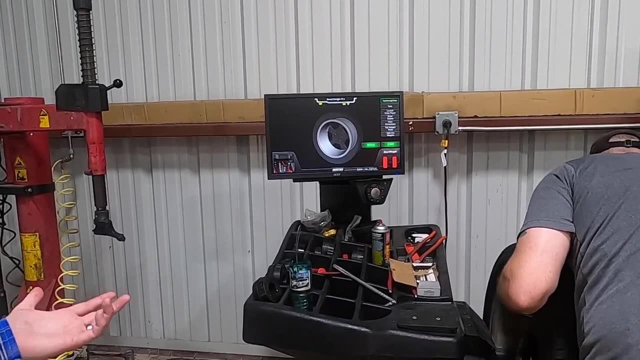 So if you look over here see this computer screen. So many things are done by computer. Even working on your tires is done by computer And that machine is going to read how the tire is balanced and it would tell you if it needs a weight on a certain side so that it'll spin more true to a circle. 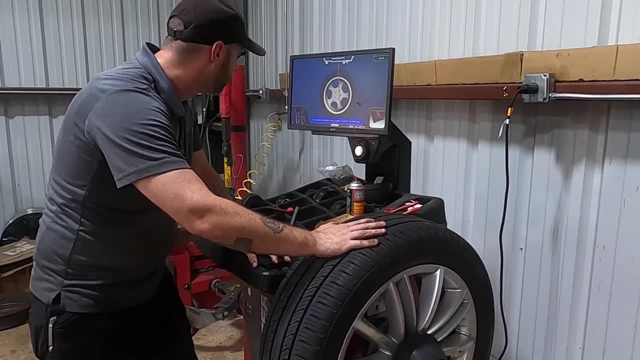 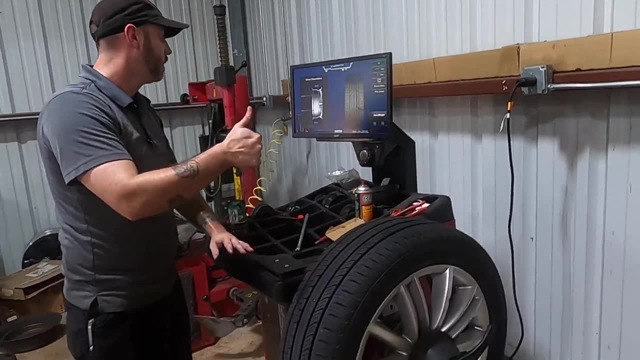 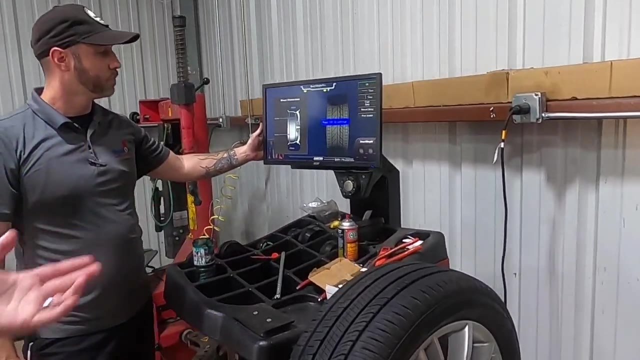 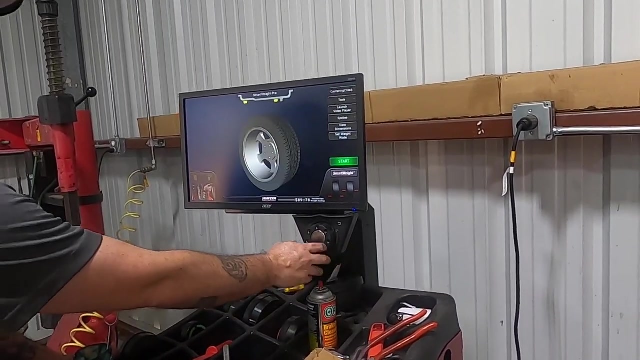 So what he did there is he was lining up the spokes of the wheel with the knowledge of the computer, so it'll all talk together. That way we get our wheel dimensions. Oh wow, That's really cool. Now it's going to measure the imbalance. 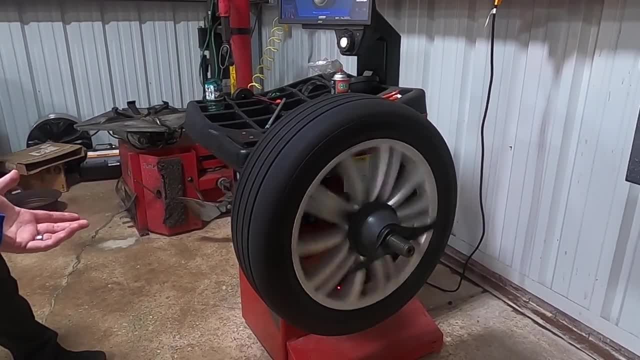 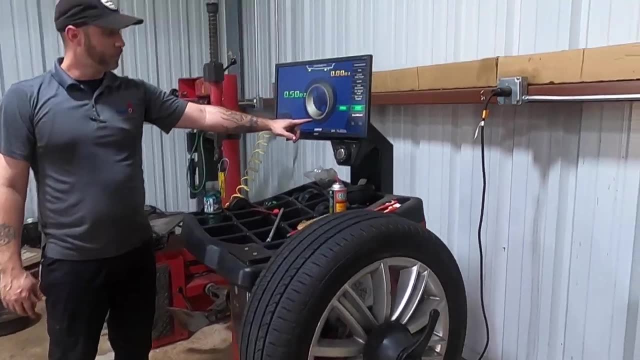 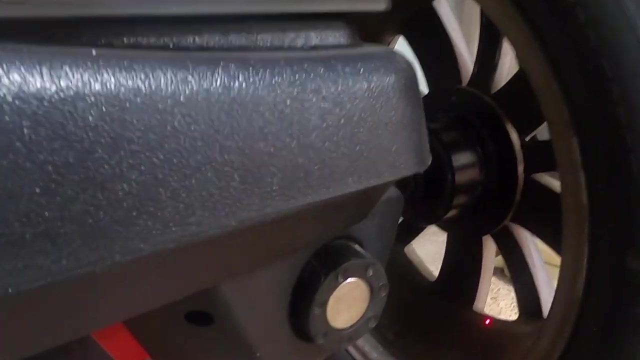 Look at that, guys. So it's spinning it and it's measuring the balance of the tire. So when it tells you to put one down, you just line your laser, which, if you want to come to this side, you can see it a little bit better on the inside. 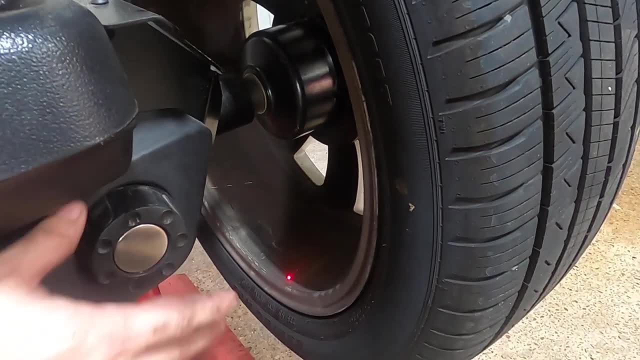 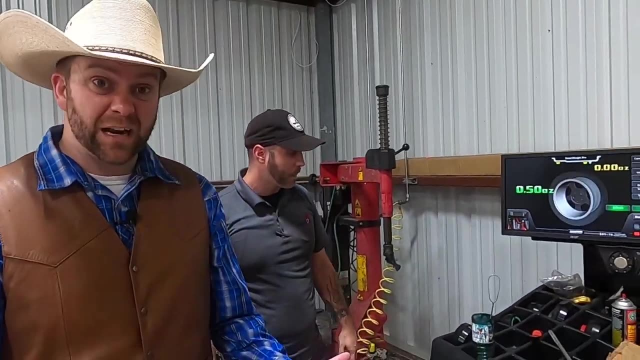 Line your laser to where it links. That's where you put that weight. Wow see, So the computer's telling Brian that that tire's a little bit out of balance and it could use a little help from a weight, And the laser's now telling him where he should put that weight. 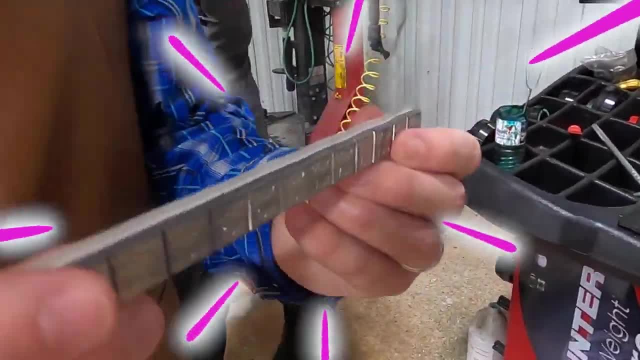 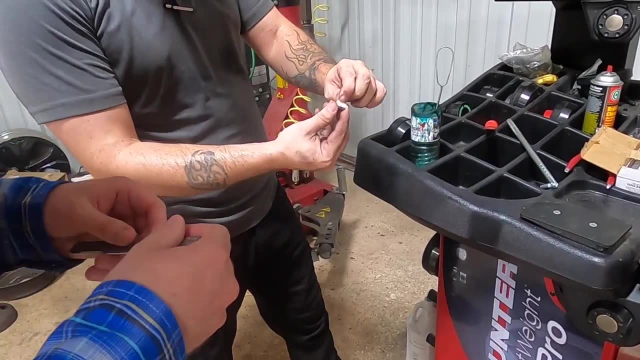 What do those weights look like? Could I see one? Absolutely Wow, look at that. I mean, they're just little pieces of metal and you're literally sticking those on the inside of the tire and it helps it stay balanced. That's really cool. 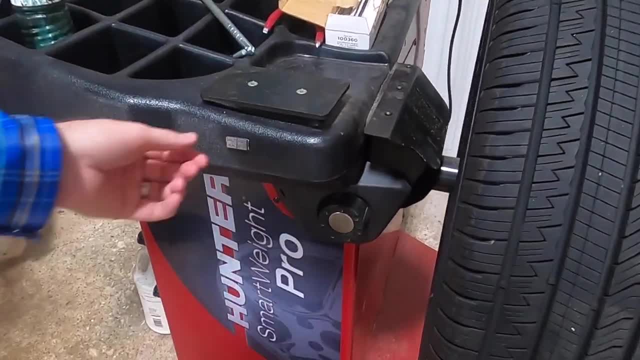 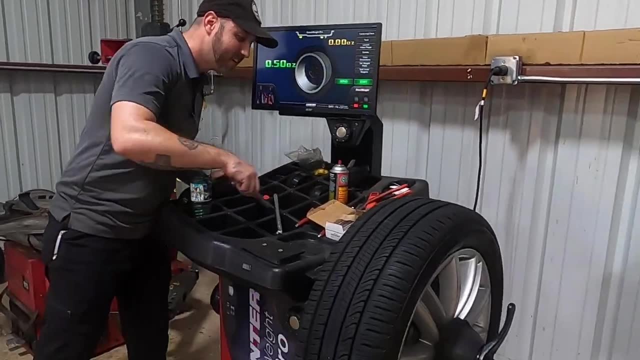 It peels off and just sticks. Whoa, that's so cool. Hey, now your table's balanced too. Yeah, Thanks for showing us that. That was really neat. Of course, I've never seen a tire balancing machine before, Have you guys? That was really fun. 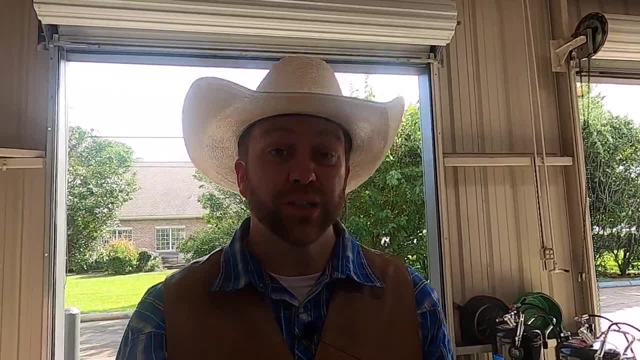 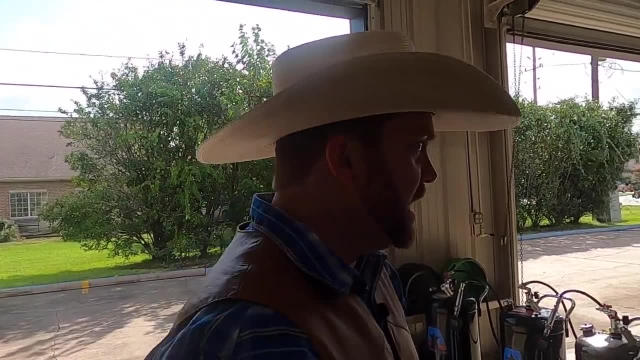 Guys check this out. So whenever you're getting an oil change, your vehicle has oil running through it. It serves as a lubricant within your motor and all the moving parts, And so every once in a while you've got to swap that oil out and keep it fresh. 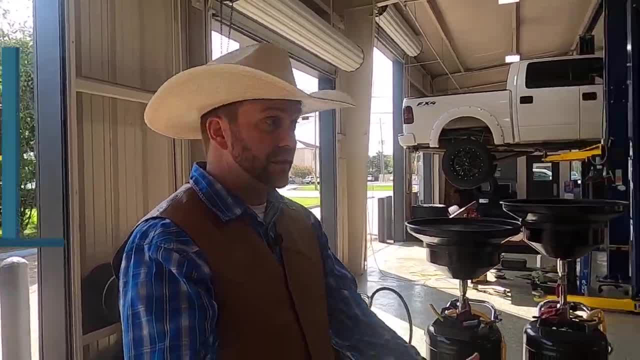 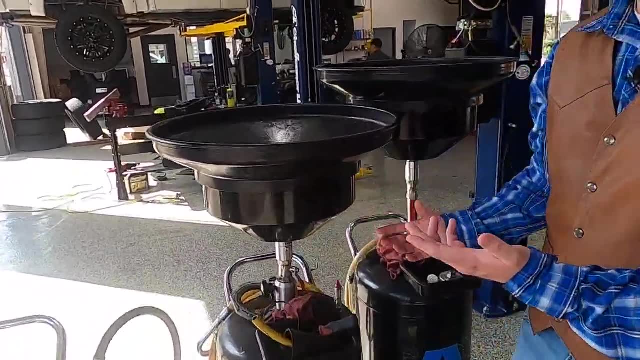 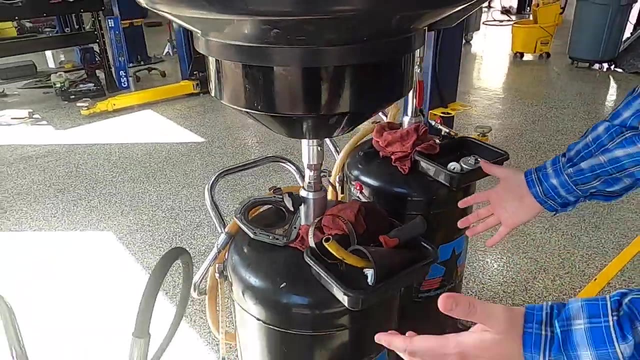 Well, what they would do is they would put your vehicle on this lift and lift it up. That way they can get up underneath it, And these right here are oil catch pans- And so they would take off your oil filter, which would let the oil that's in there run out, and it would run into this, and this is where they catch it, in this big reservoir down here. 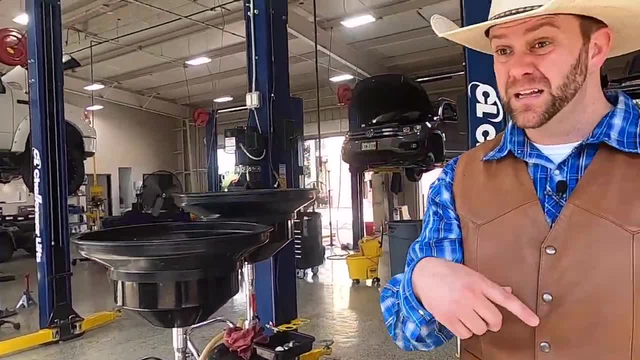 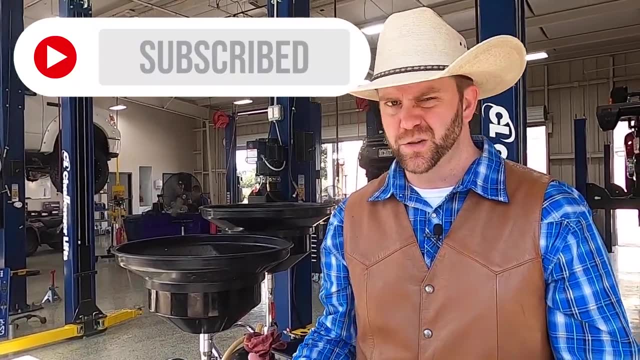 And so once the bad oil is in here, they put that in a big receptacle outside and there's some environmental folks that come take that off and make sure that it's disposed of properly, because you wouldn't want to just put oil in the trash. You can't do that. It's bad for the environment. 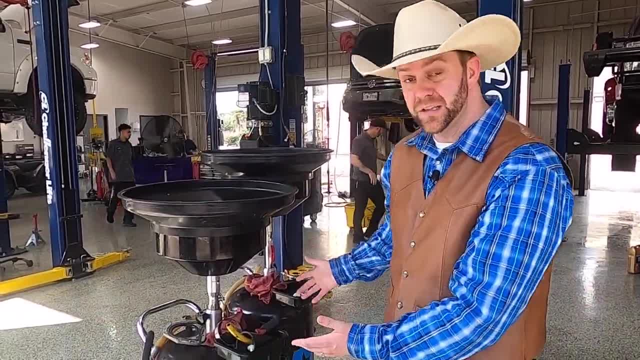 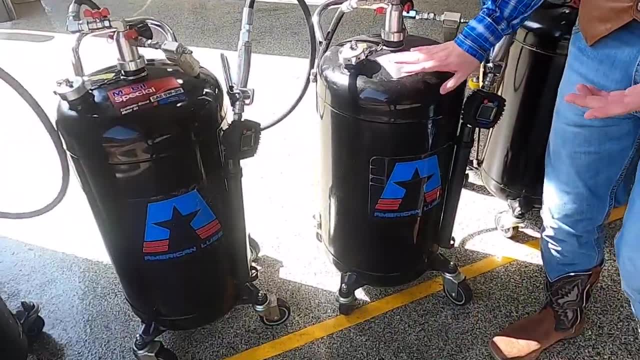 So they dispose of it properly by containing it in these vessels and making sure it goes in the correct receptacle and eventually taken care of the right way. And then they use these big cans right here. All of these are pressurized motor oil. 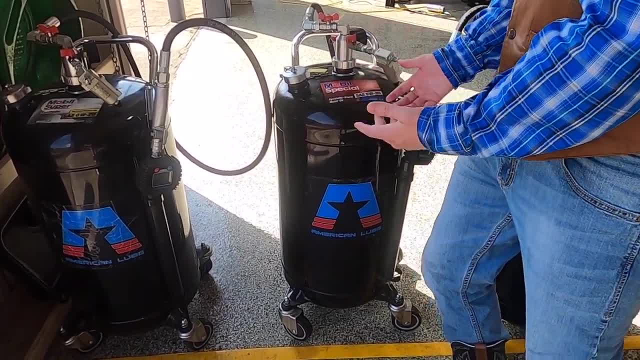 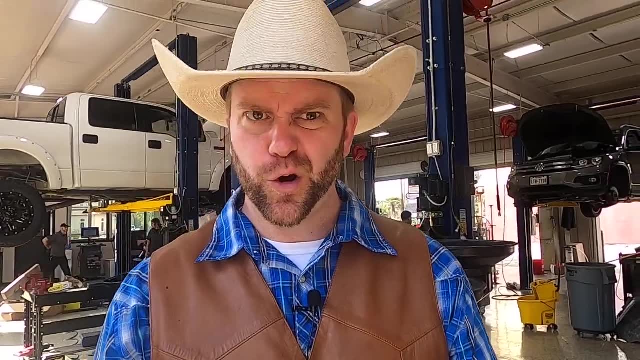 And so they take there's brand new oil in here and you pressurize it with air and then they can use that to fill your car back up with oil. That's like a really simple description of an oil change. There's a lot of work that goes into it and they check a lot of other things on your car while they're checking your oil. 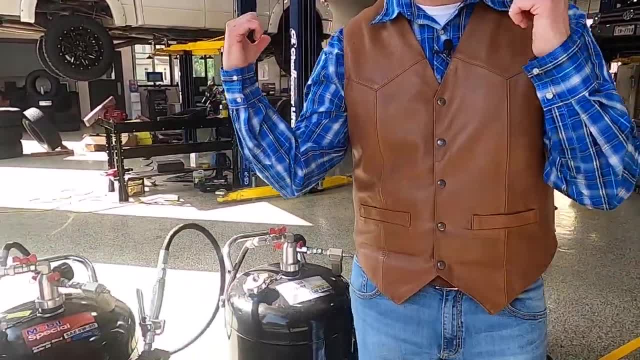 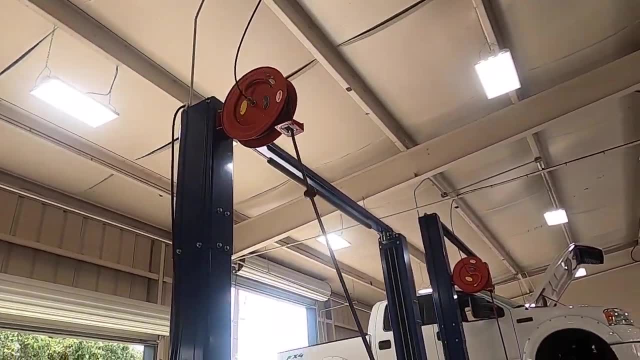 But I just wanted to show you these big oil containers and the catch pans. That's really cool, And, guys, another thing you see around this shop is these right here. You see that thing on a big reel up there. You guys know what this is. That's an air hose. 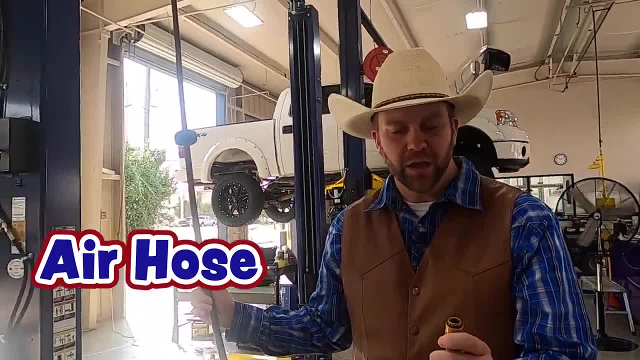 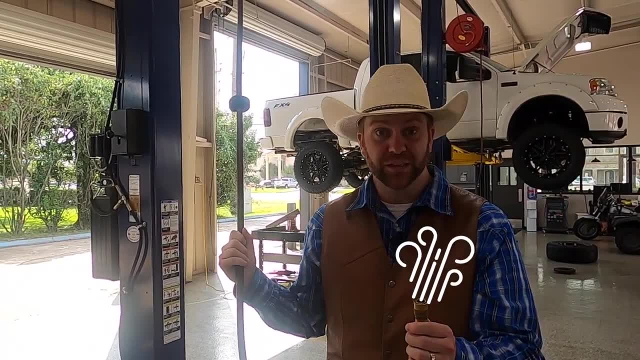 They use compressed air to blow a lot of things around in the shop. So if a tire is a little bit low, they can use this air pressure to fill it up. Or they also use something called torque wrenches or impact wrenches, and those are powered by air. 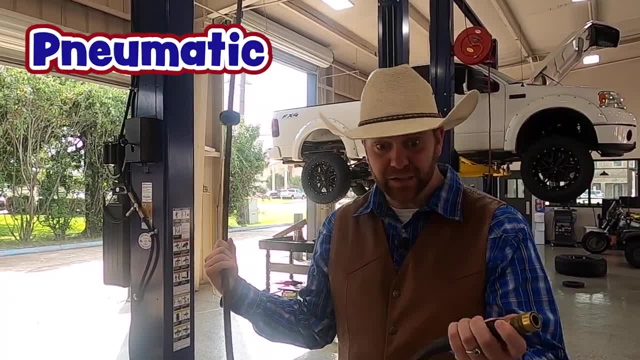 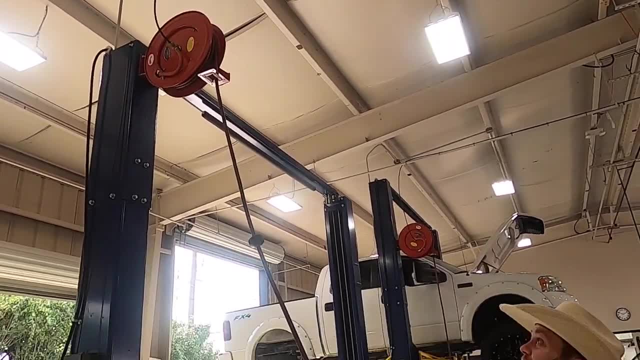 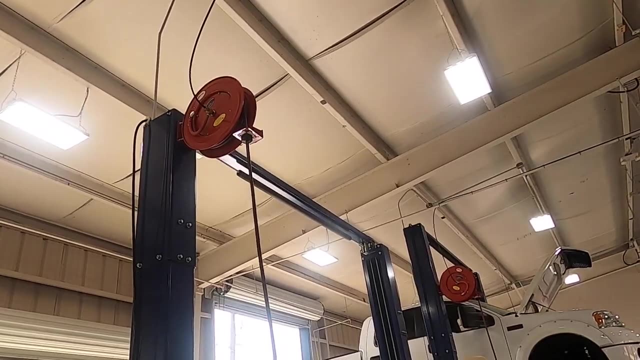 When something's powered by air, it's called pneumatic, And so they use compressed air that comes through these big hoses all over the place to use those tools. That's really neat. See, it's got this right here. This is cool because when you let it go, it stops it right up there at the top, so it doesn't go any further. 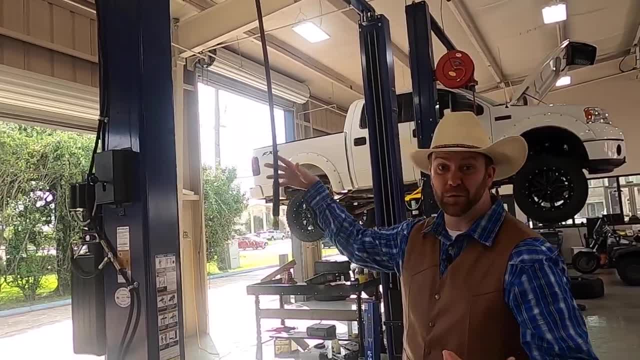 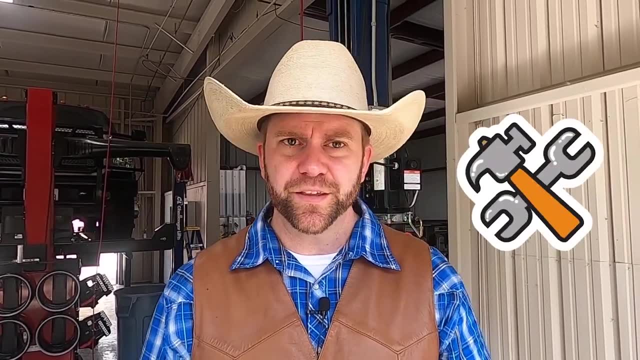 So you can always reach the hose. If that wasn't there, it'd reel up all the way and you'd have to be really tall to grab it. Hey guys, you know what mechanics have to use. They have to use tools all the time. 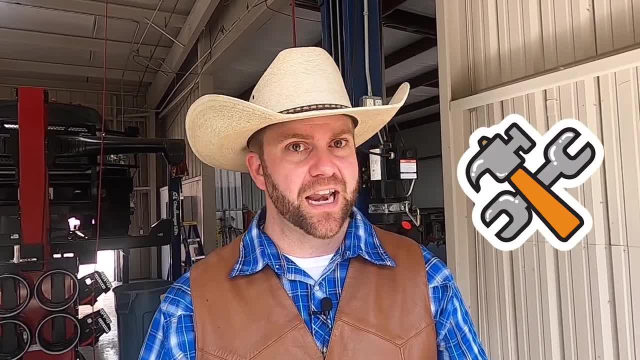 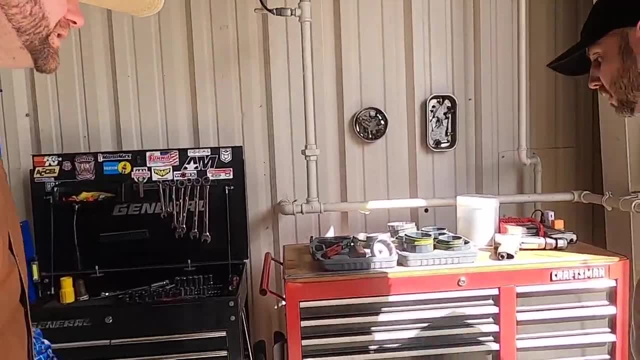 They're always using tools, and so it's important for them to be organized and have a spot for everything Brian's offered to let us take a look at his tools, because I'd like to learn about what kind of tools they use. All right, so in this top drawer it's going to be all of our screwdrivers. 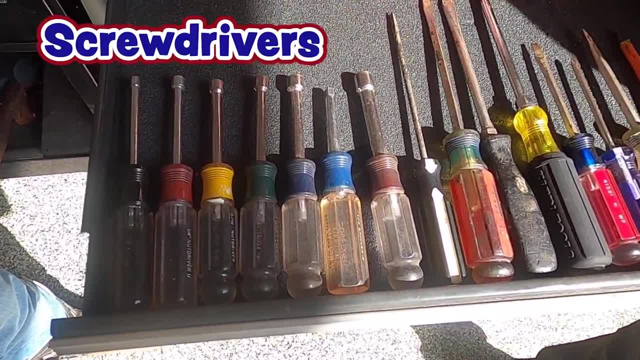 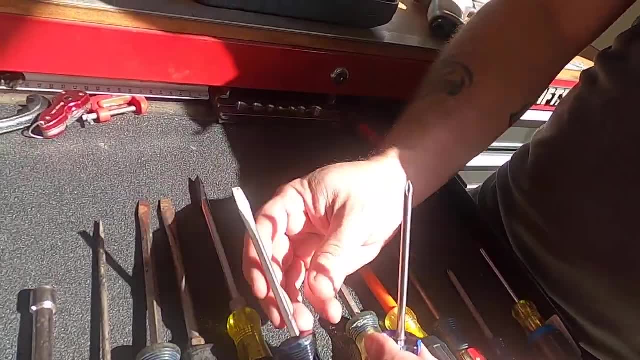 We also have nut drivers here for different sizes, and then our screwdrivers for different applications: different lengths, different sizes, different tips. Wow, Phillips head and your flat head to be the two main differences. So I know this. I'm not real good with this. 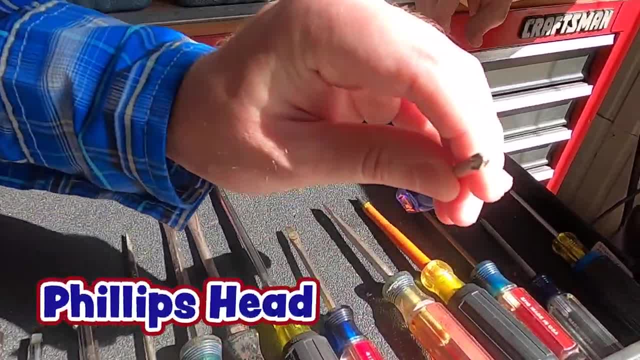 I've never used any of these tools, but I know this one's a Phillips head, this one, that's all pointy like that. and then the flat head is really simple to figure out. because they call it a flat head, because, look at it. 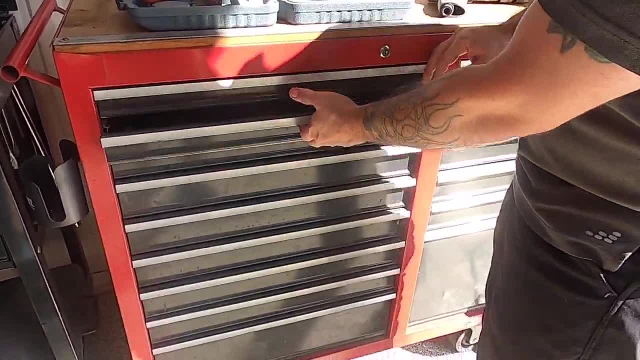 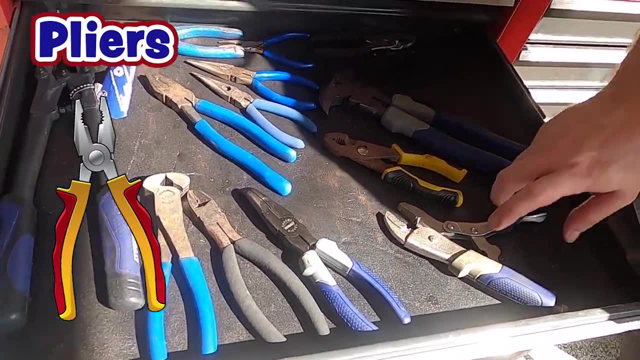 It's got a flat head on it, All right. moving next, this will be all our different types of pliers we use. We have needle, nose, crimpers, cutters, vice grips. That's a whole bunch of pliers. 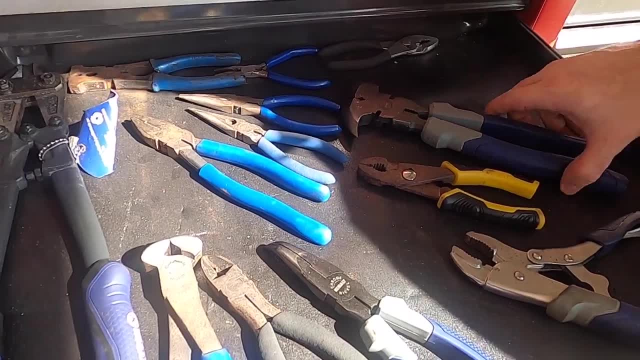 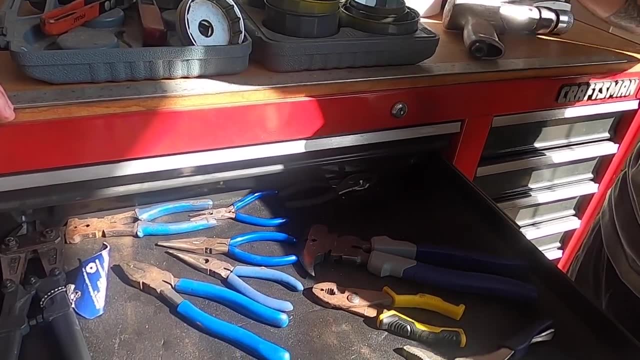 Absolutely Wow. this one's got something sharp on the end of it Every now and then. this one gets used for a lot of different things. Its most usage is barbed wire for fencing and sometimes we have to do work exterior on the building. 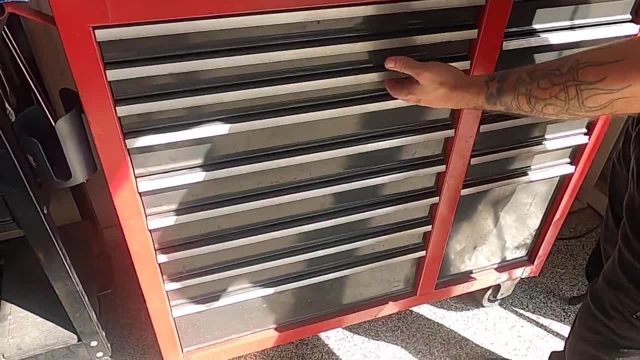 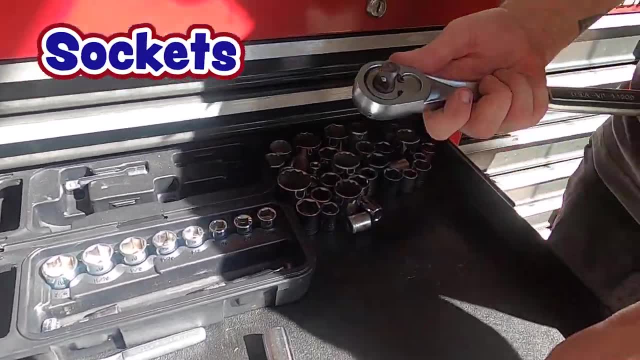 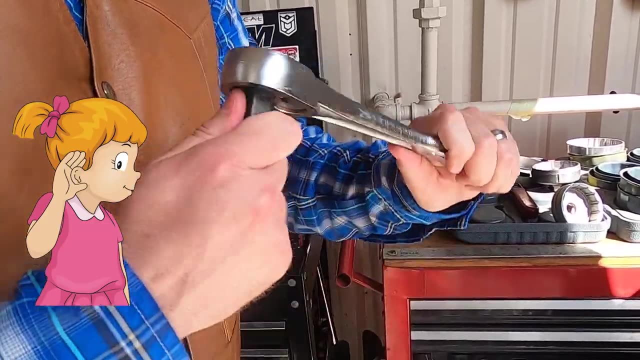 Oh, okay, Very cool All of that. We have sockets Those will fit any type of ratchet, Doesn't matter which one. Let me see one of those real quick. You guys hear this. These ratchets make a real funny noise. 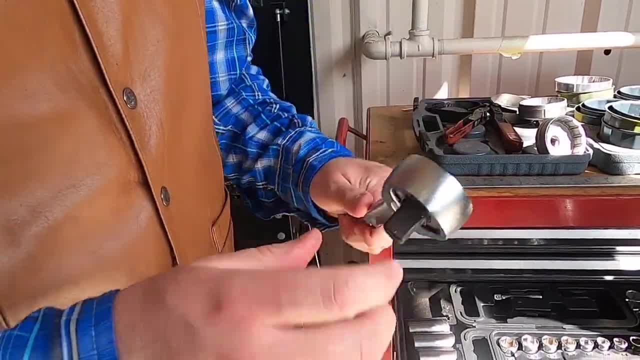 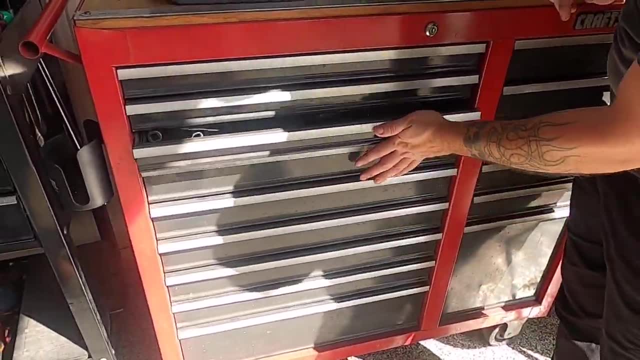 But they only turn one direction when you have it selected that way and then if you want to loosen it up, you just turn it the other way. Ratchets are really cool and I love the sound that they make. Here we have some heavy duty wrenches. 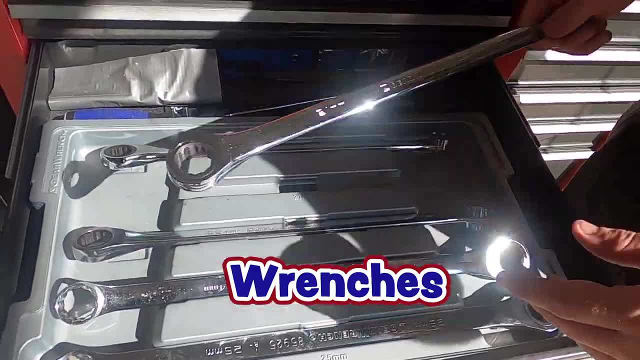 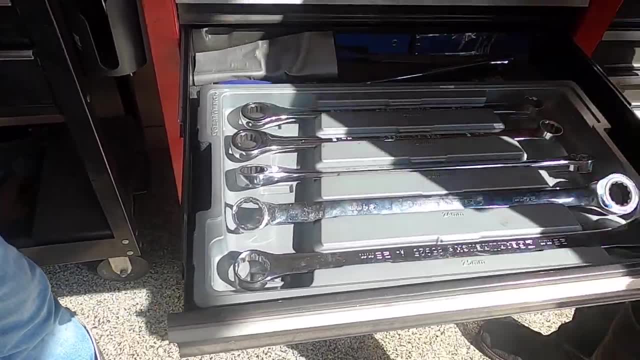 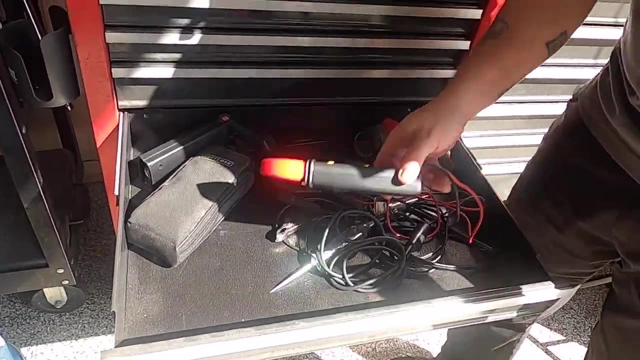 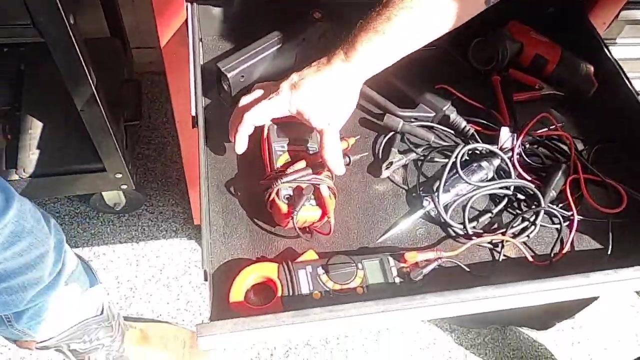 Wow, These are for our suspension work. Those are really big. These ratchet as well. Those are really neat, Wow. So we also have to do a lot of electrical testing. Wow, electrical testing. I forget that cars even have electric systems in them. 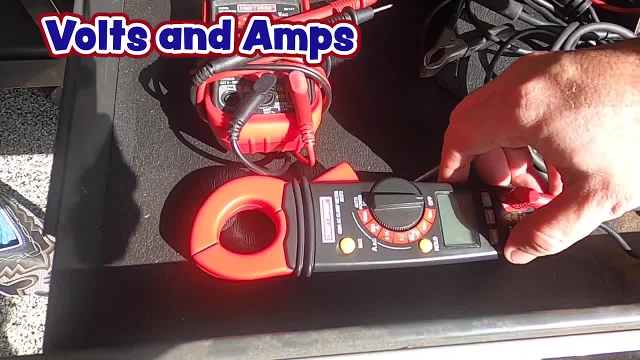 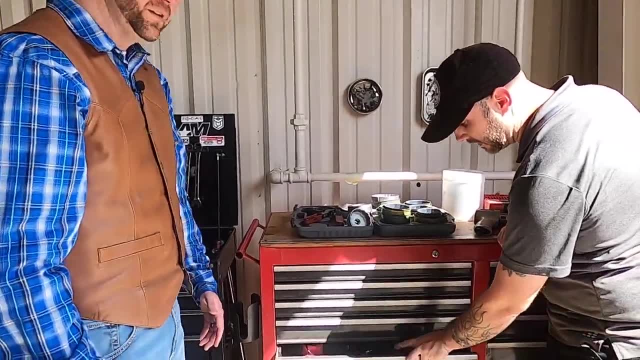 This here tells you volts and amps on cars. This just tells you amps. Wow, You have to know so much to be a mechanic. That's a really skilled trade. Absolutely, That's so neat. Whoa Heavy duty wrenches. 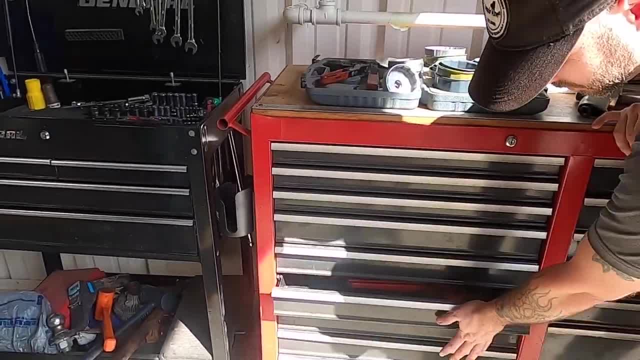 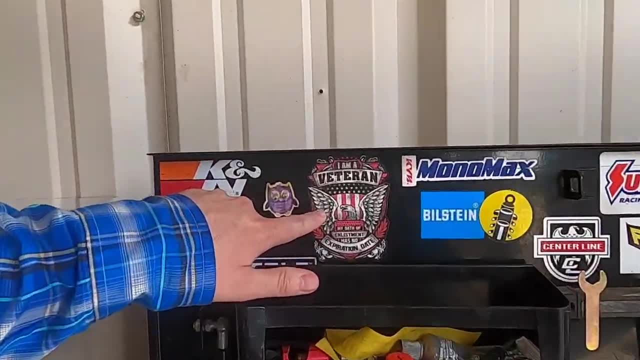 Big, big wrenches. All right Here, let's see. This is another area that you keep some tools. Hey guys, check out this sticker that he's got right here. Y'all see that It says I am a veteran. 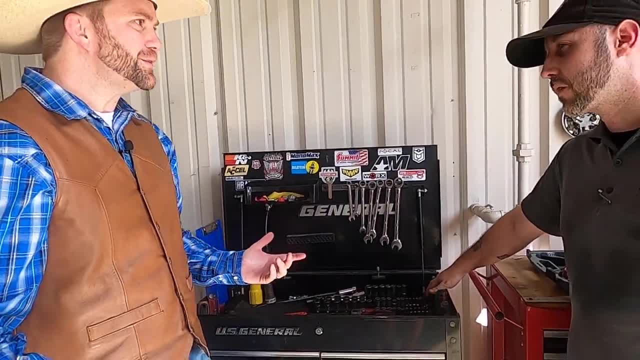 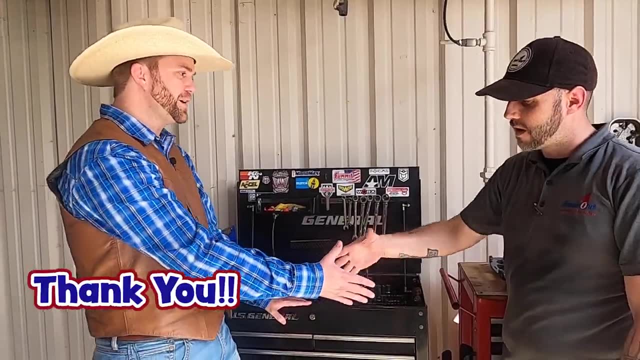 Wait a second, You're a veteran, Absolutely. Where did you serve? I served pretty much all over, but San Diego, Okinawa and Iraq, Wow, Well, hey, thank you very much for your service. I appreciate you keeping us safe and everything you did for our country. 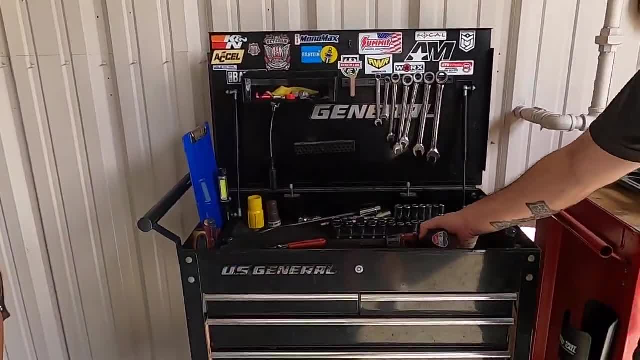 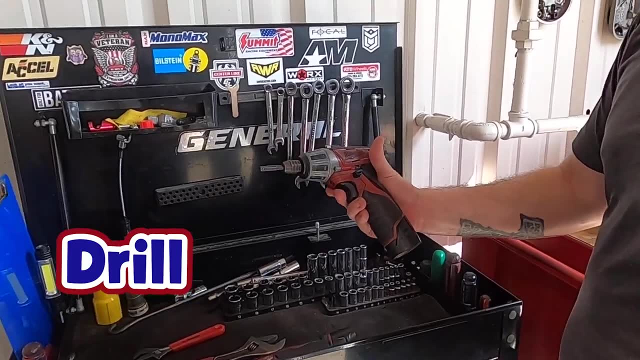 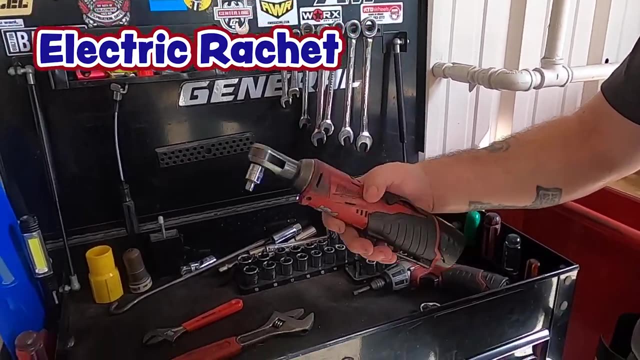 That's so cool. Anyways, all right, Sorry. What about these tools? So here we have battery operated tools. You have your drill, Which works any direction, And then your electric ratchet. Oh wow, I've never seen one of those before. That's really neat. 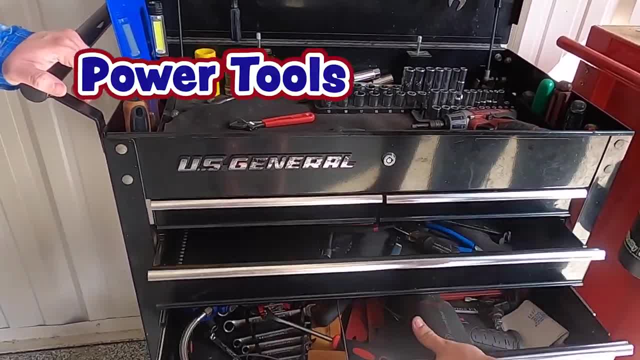 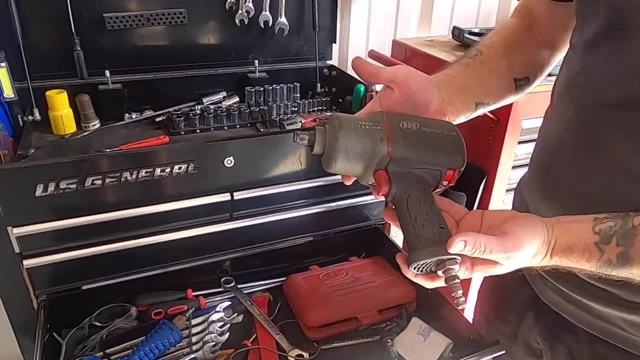 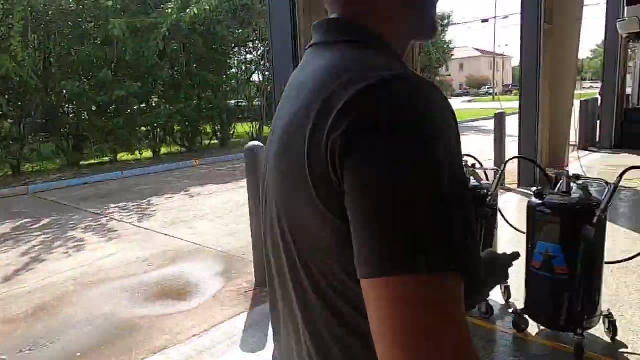 And then in here we have our power tools. So here's an air impact And how that works. I will show you how that works with the tire filler. Wow, Let's go check that out. Look, he's using that air hose that we talked about. 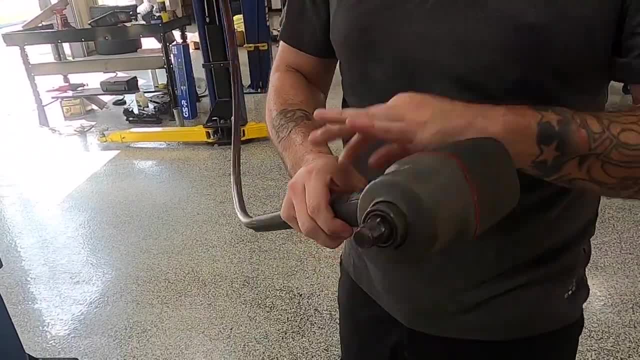 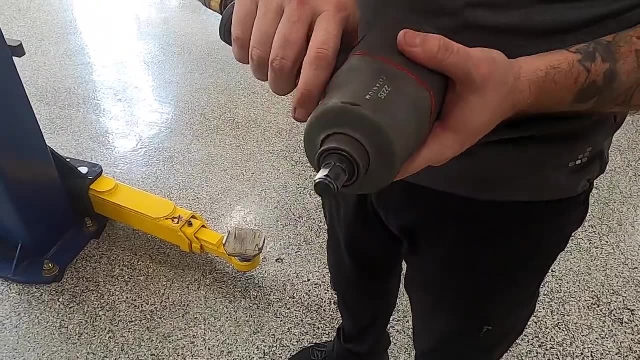 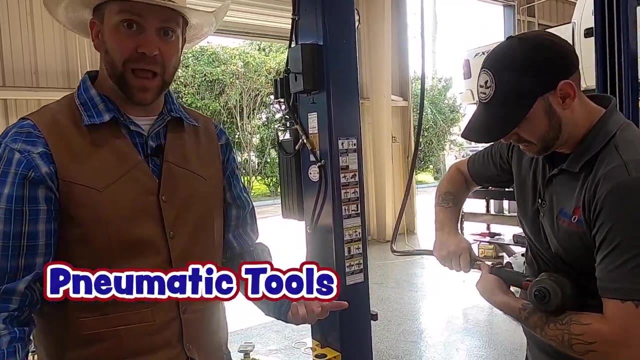 Feel that back, Make the two surfaces, And then that works different ways. That is so cool. So this is one of those pneumatic tools I was telling you about. It's pneumatic because it's powered by air. That's really neat. 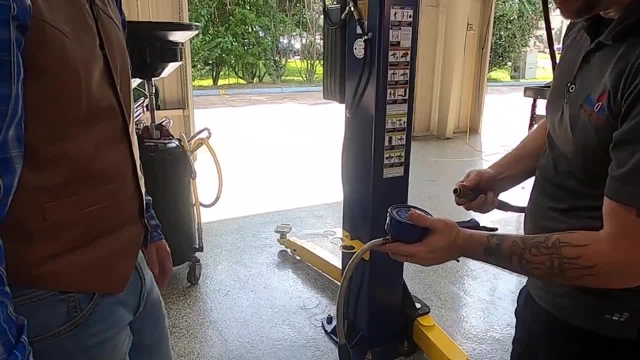 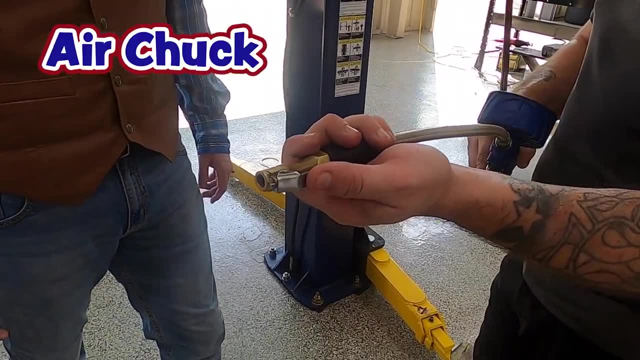 And then this is what you use to fill your tires with air. What is this? This is what you use to fill your tires with air. We call it an air chuck. An air chuck. Okay, So you will put it onto the threads which you will have to clamp onto your tire. 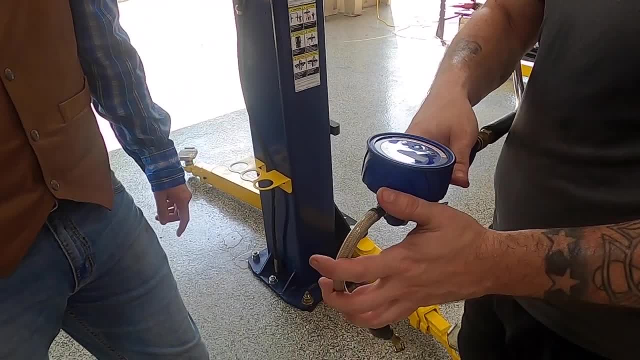 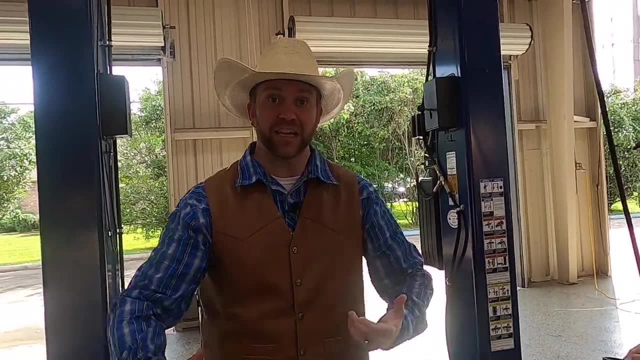 And that tells you how much pressure you've got in the tire. That tells you the pounds per square inch PSI. Wow, I didn't even know that's what it stands for. So whenever you're looking at a tire, it's got a number on it that says X amount. 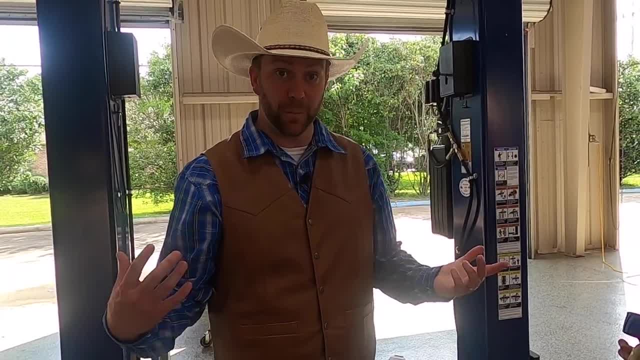 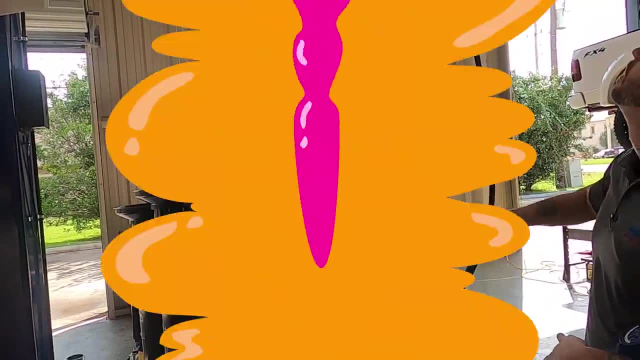 PSI Brian just explained to me that that stands for pounds per square inch. That's really cool, Absolutely Wow. You know, working on cars can be a dangerous job. There's a lot of things you have to do to stay safe. 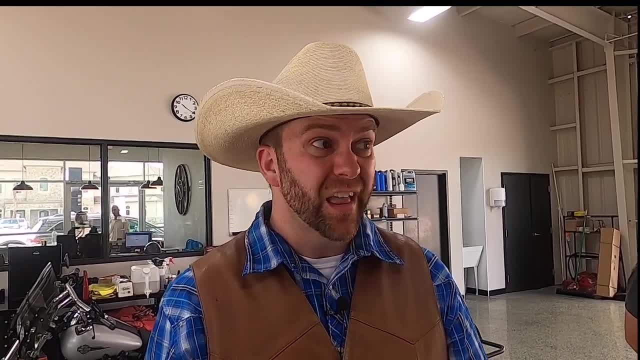 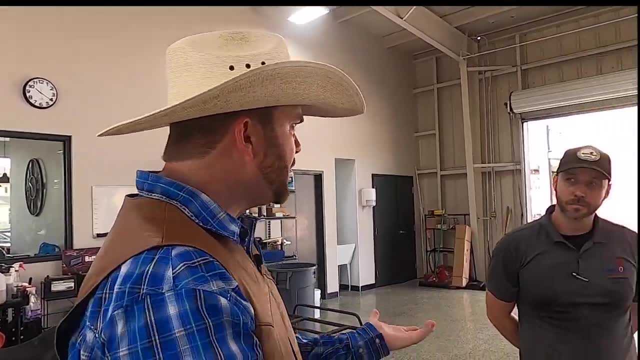 Like we talked about. you wouldn't normally just walk right underneath a vehicle, And there's also a lot of times if you're working underneath a car and you're looking up, things could fall in your eyes. That wouldn't be good. So you wear. what do you wear? 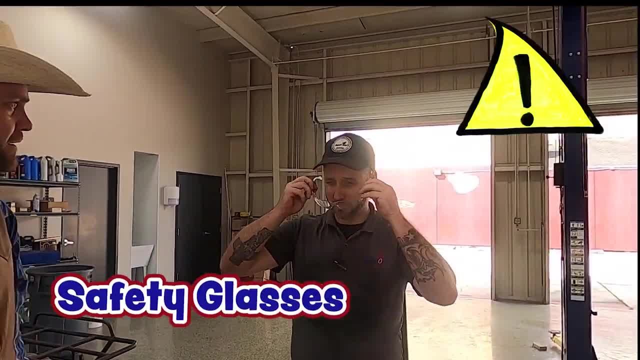 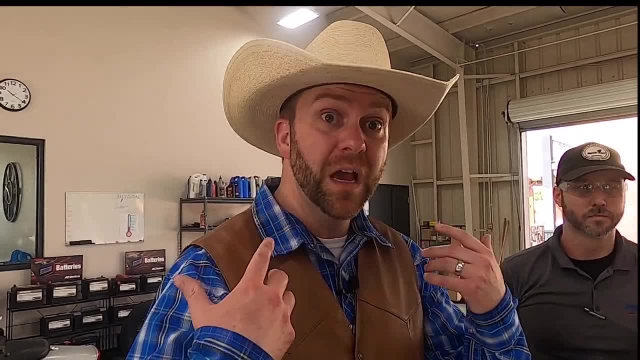 So we do have safety glasses. Okay, We all have to wear them, Just like that, See. And safety glasses keep your eyes safe so nothing would fall in them. And then they also have something really neat. Do you guys see what this is right here? 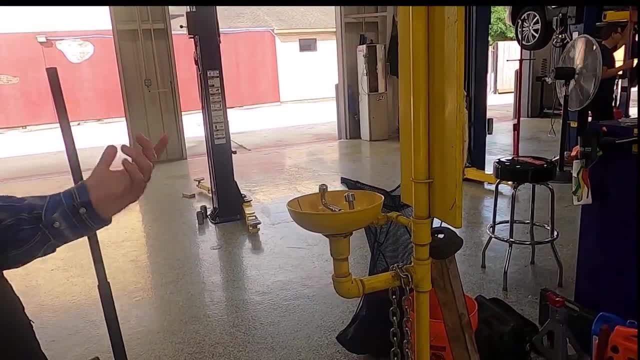 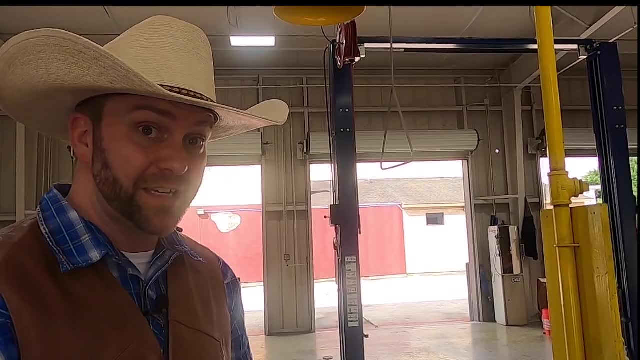 Hopefully you don't already know what it is, But I'm going to tell you. This is called an emergency eye wash station And they have these in a lot of different facilities. This auto shop goes the extra mile about safety because they actually have one here. 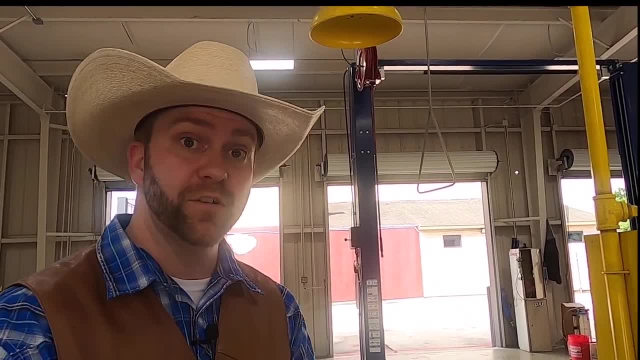 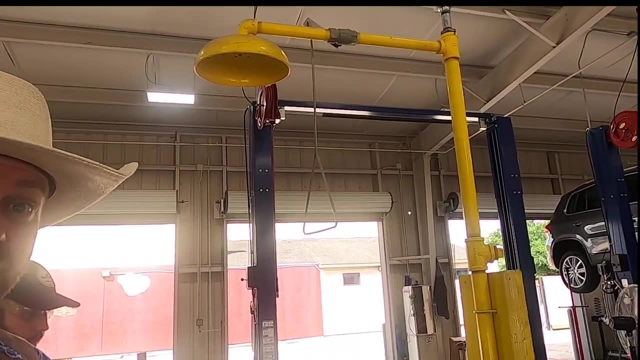 Most auto shops don't even have those, But you'd find these in chemical plants, in pharmaceutical facilities, even some dairy and food processing plants- Any kind of atmosphere that heavy work is going on. they have emergency eye wash stations And what this is- if you got something in your eyes, that was really, really bad. 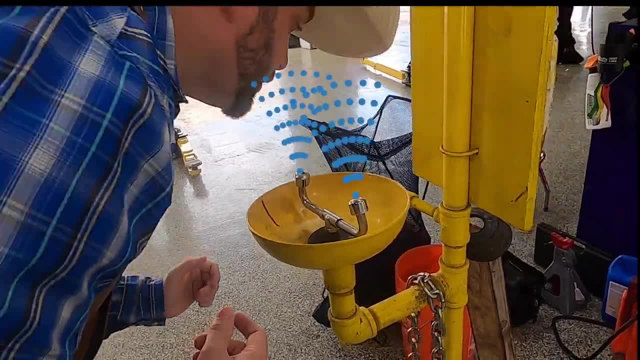 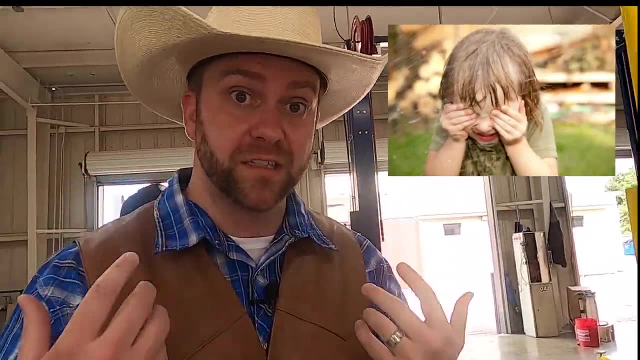 you would come over here and I'll just show you. You would put your head down like this and pull this lever right here and it sends a big rush of water so it splashes in your eyes and washes out whatever's bad in there. 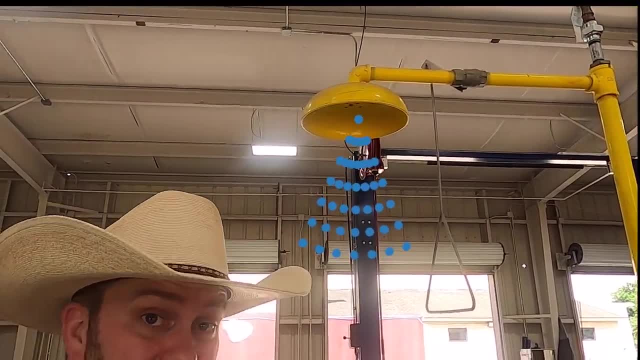 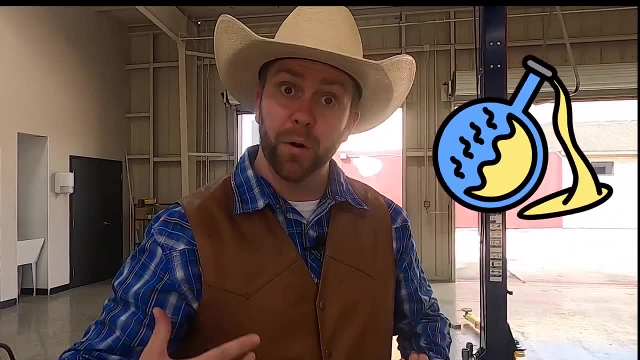 And also this has just a safety shower. A safety shower is the same concept, except it's not so big And specifically for your eyes, if you were to get a chemical spill on you or like a burn or something bad happened, you wouldn't have a chemical spill that could hurt you here. 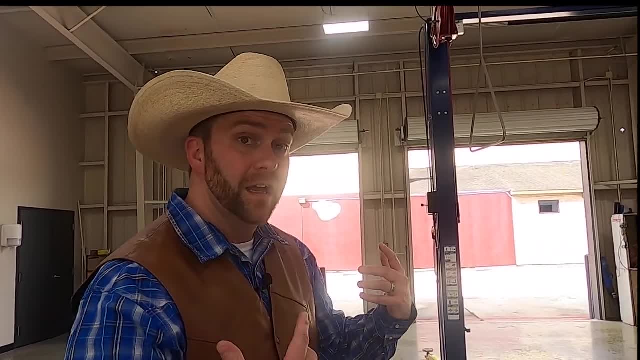 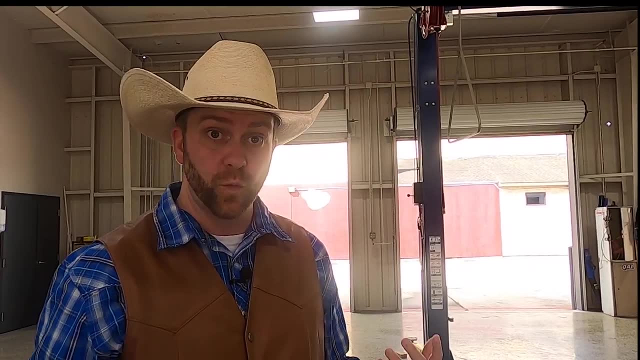 because there's no chemicals that could really hurt you bad here. But in a chemical environment you would pull this and it would rush a lot of water on you And you would stand under that for a long period of time to wash all those things off of your skin. 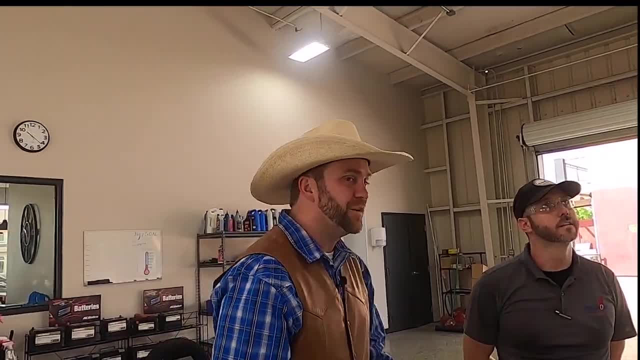 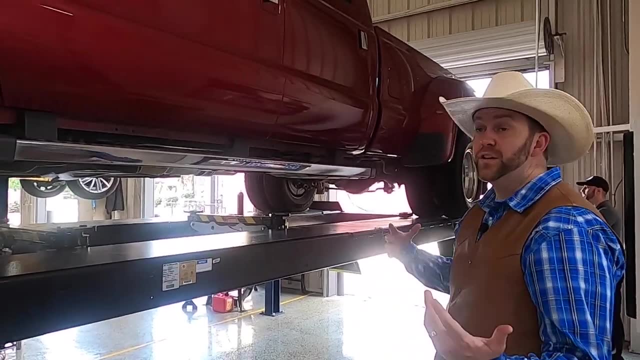 That's really great that you all have that and take the extra mile for safety, Absolutely Wow. What a proactive way to run your shop. That's so neat. So there's all kinds of different lifts. This is a really big lift because you see what's on it. 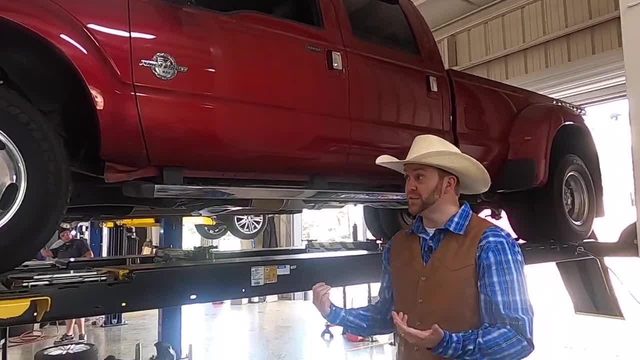 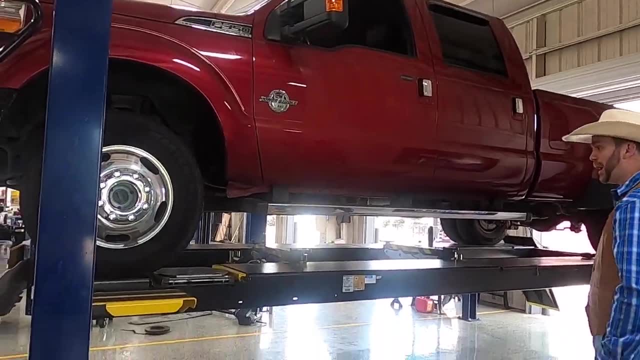 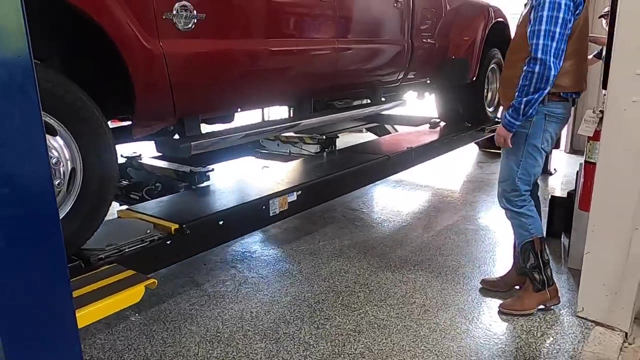 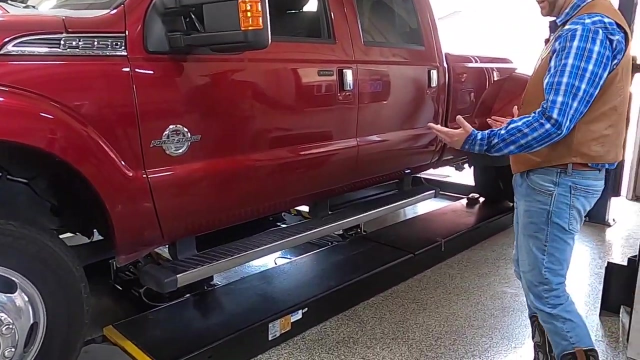 A really huge truck. Brian said he could show us it in operation. Look, it's already going up, Now it's coming down. Wow, that's really neat, Boy. that's so, so cool. And now the truck is all the way on the ground. 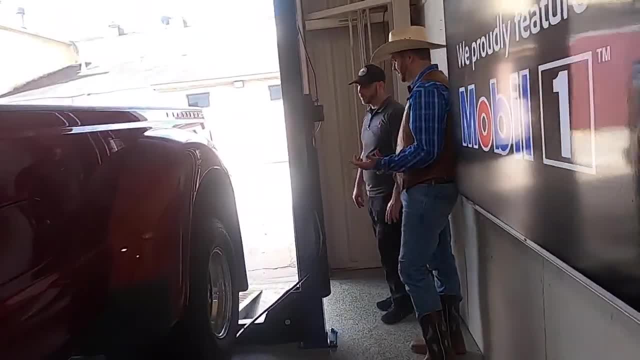 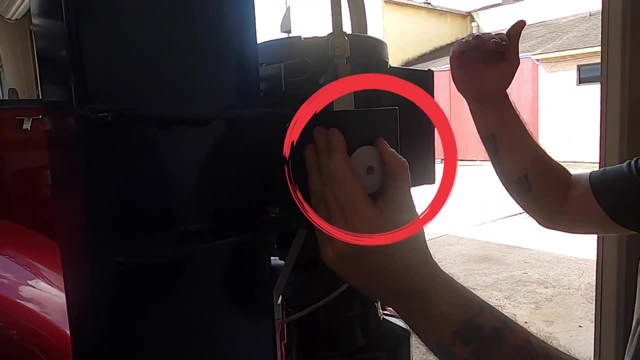 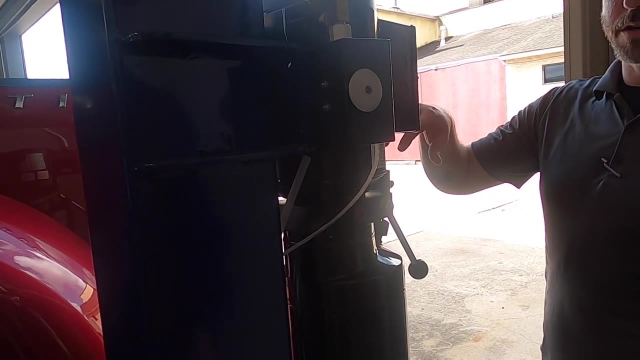 So you just use these different controls over here to do that Absolutely. This control here applies or not, applies the brakes and or locks, This one lowers it. So would this be full of hydraulic fluid here? Correct: This button here controls the electric generator, here motor. 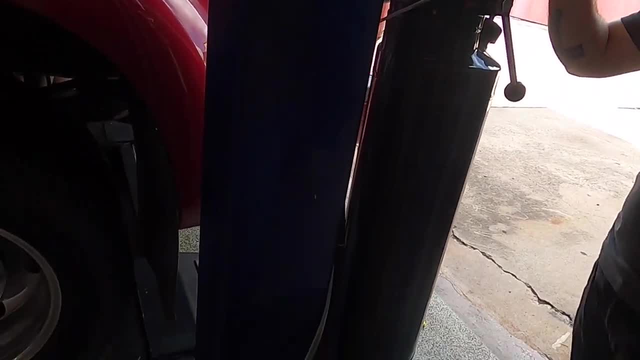 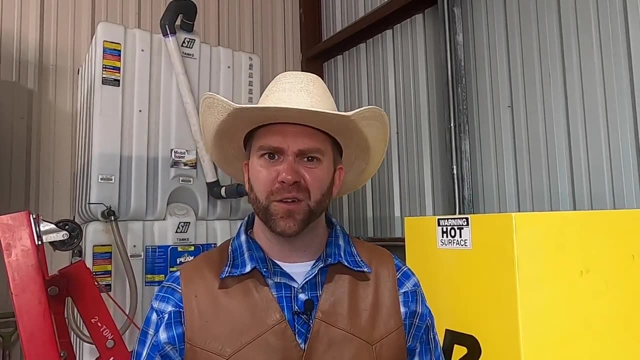 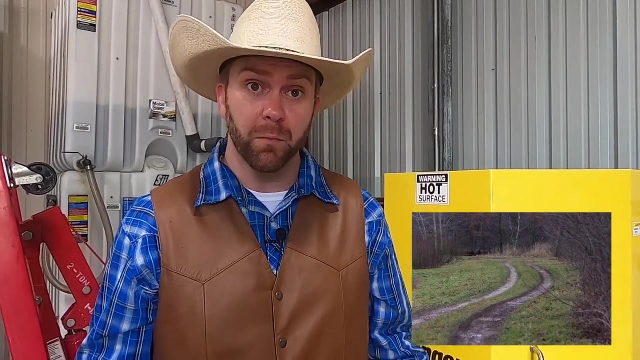 that moves this fluid throughout the lines. Wow, Hydraulics at its finest. That's really neat. All right, guys. Well, you know, cars run on the road. What is the road? It's really dirty. There's all kinds of dirt and grime and oil and other debris that comes up from the road. 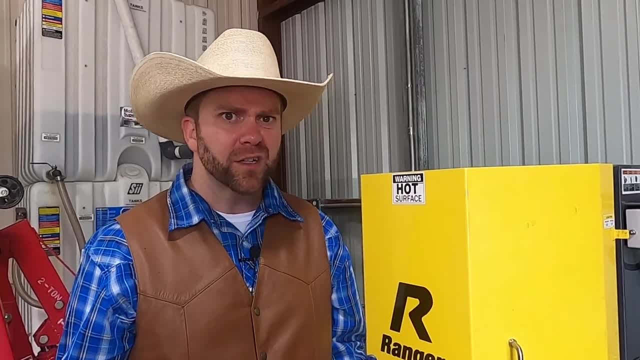 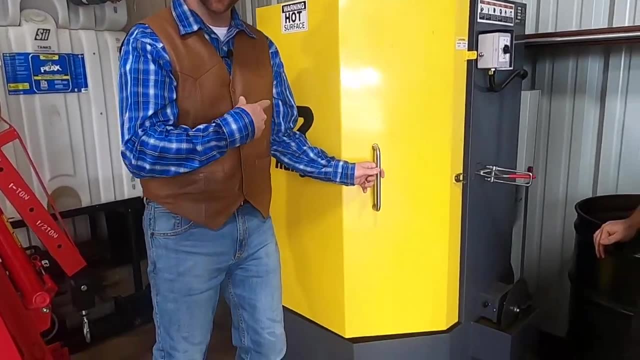 into your engine compartment and onto your vehicle. So whenever they're working on cars, there's a lot of things that are really, really dirty. What do they need? A big old parts washer. That's what this is. It doesn't look like a sink, but this is an industrial strength parts washer. 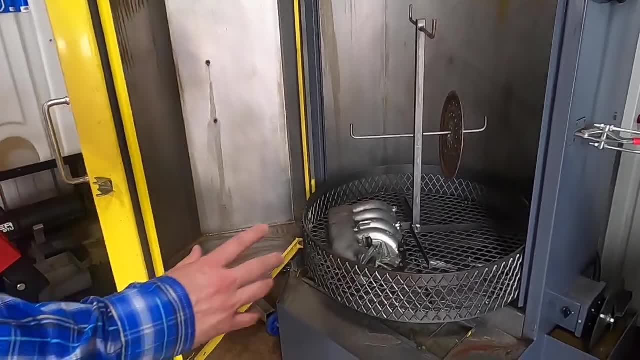 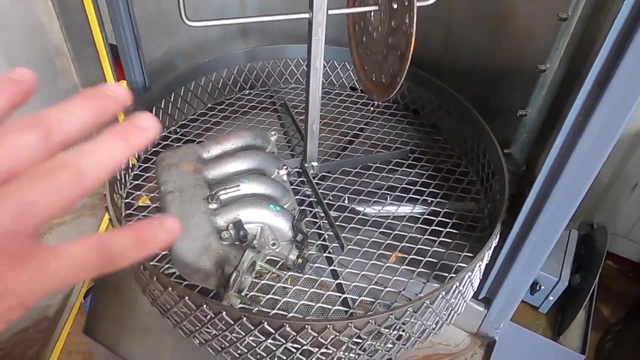 Let's open it up and take a look. Wow. So it's got all this little- I don't know what you would call this- some kind of tree to hold different parts on, And you put those in here And as soon as they're situated, you can close it up and it'll wash them for you. 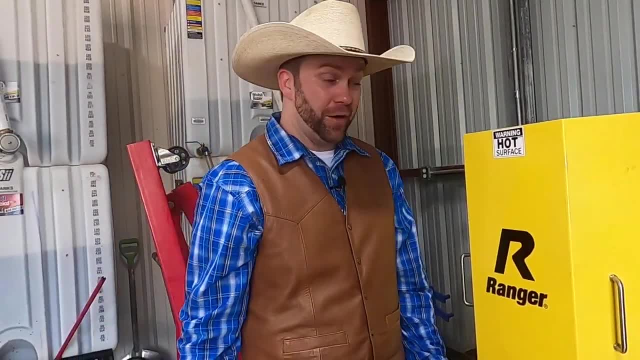 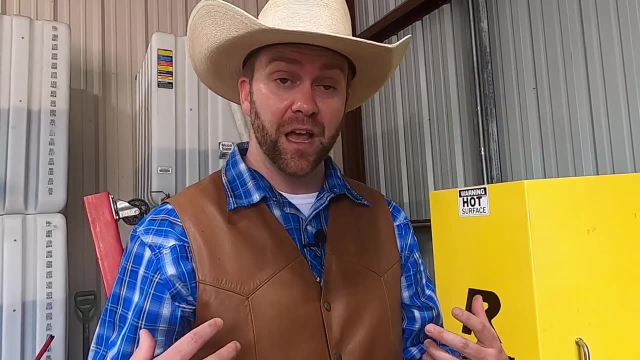 Whoa, You hear it starting up. That's really loud. I bet there's all kinds of water splishing and splashing all over those things. There's also some chemicals used to make sure that all the oil and debris gets taken off of there. 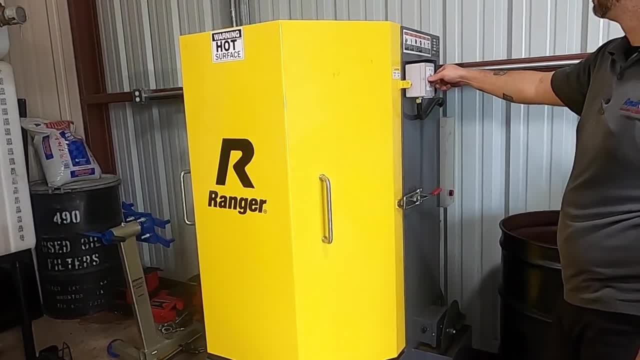 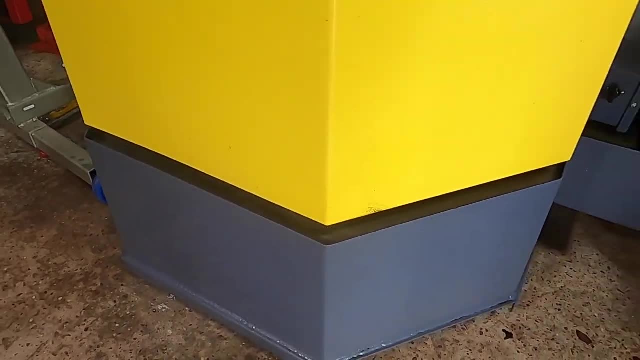 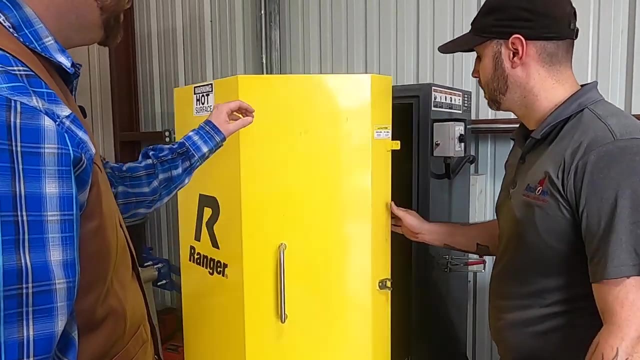 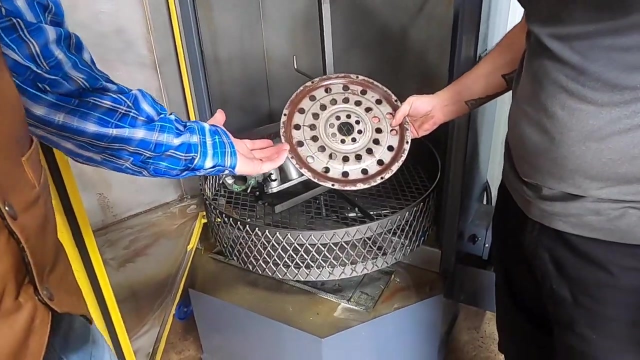